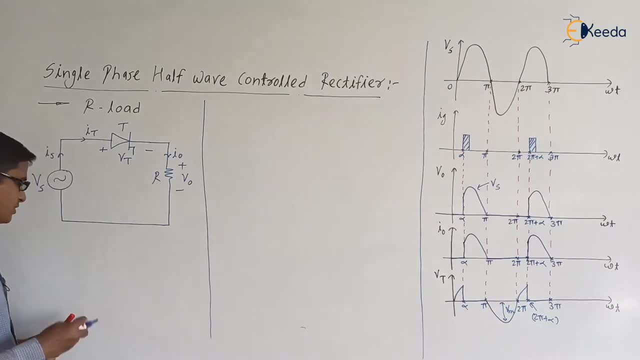 Supply voltage. Vs is equal to Vm into sin of omega t, So here Vs is equal to. So here Vs is equal to Vm into sin of omega t. Vs is equal to Vm into sin of omega t. So from omega t is equal to 0 to pi, Vs is positive. 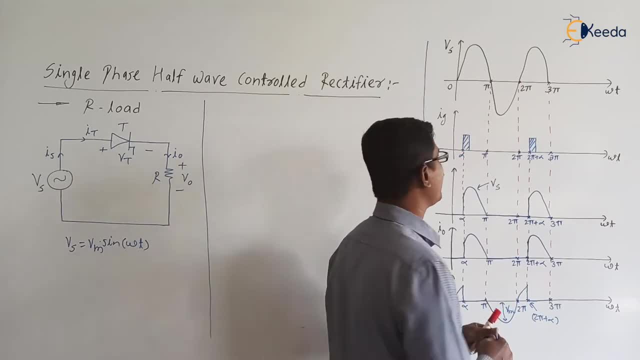 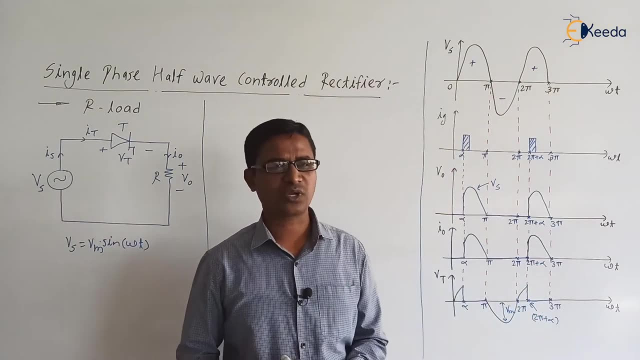 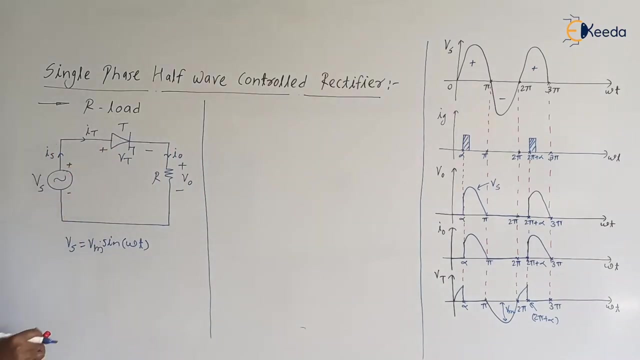 From pi to 2 pi, Vs is negative. 2 pi to 3 pi, again it is a positive. So here Vs, we are having the positive, negative, positive and negative pulses, or the values Next. So suppose if Vs is positive, the polarity will be plus here and minus here. 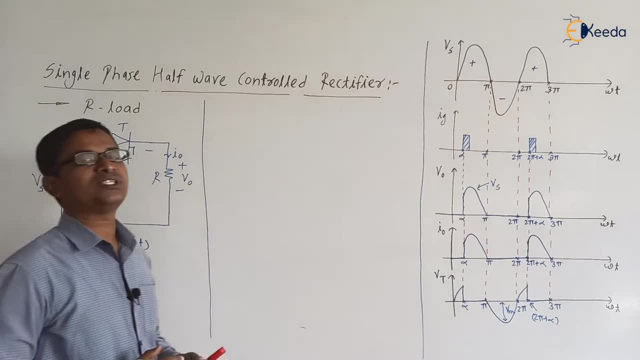 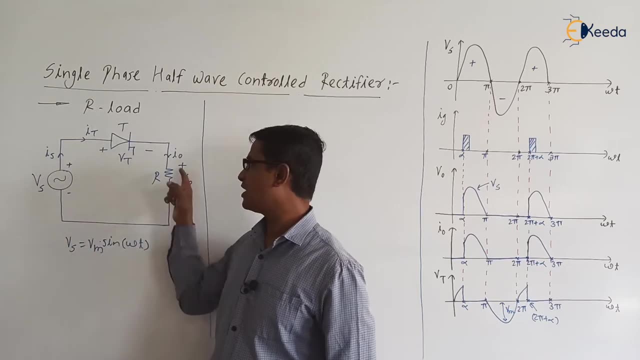 So this is like a highest potential point in the circuit. This is like a lowest potential point in the circuit. So if you check when Vs is positive, the highest potential is appearing at the anode of thyristor. Lowest potential is appearing at the cathode of thyristor. 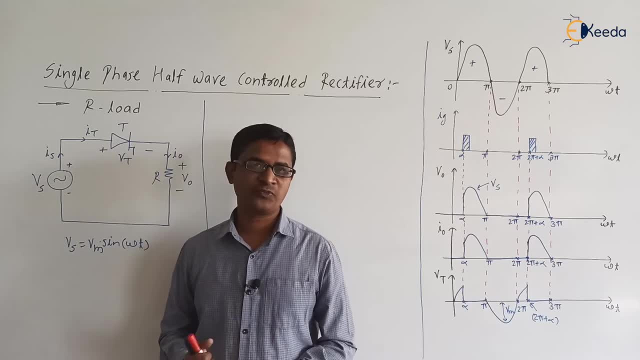 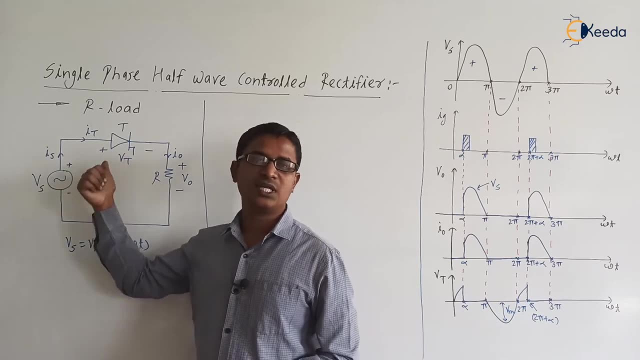 So can we say that anode is at more potential than that of the cathode. So thyristor will be in the forward bias mode. So please, important to note. Point to be noted: When Vs is positive: yes, the thyristor T will be in the forward bias mode. 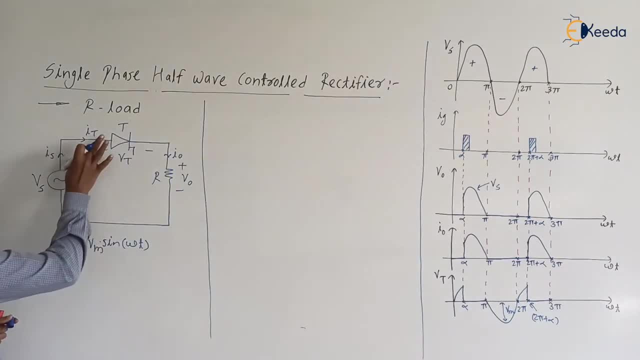 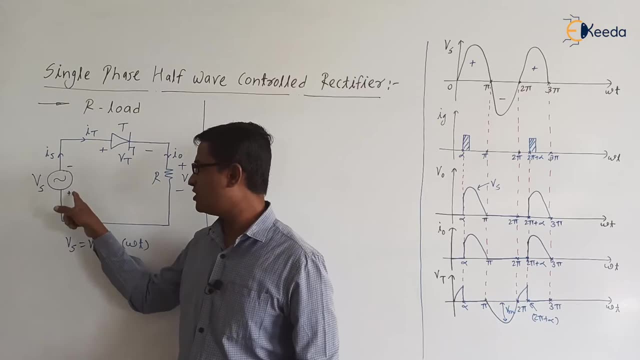 Similarly, when Vs is negative. when Vs is negative, yes, here it is a minus and here it is a plus. So, when Vs is negative, this is the lowest potential point. This is the highest potential point. Lowest potential is appearing at the anode of thyristor. 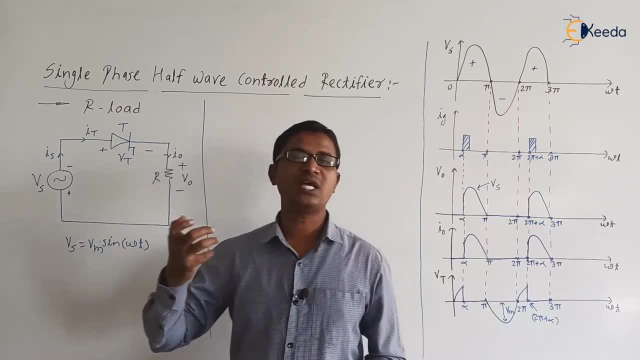 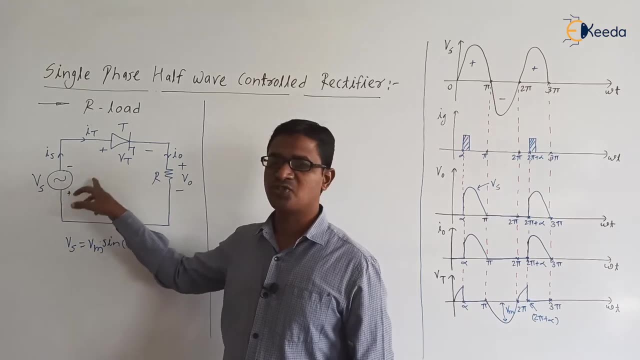 Highest potential is appearing at the cathode of thyristor, So anode is at lowest potential. So therefore can we say that the thyristor is in the reverse bias mode? Yes, So when Vs is positive, thyristor T is in the forward bias mode. 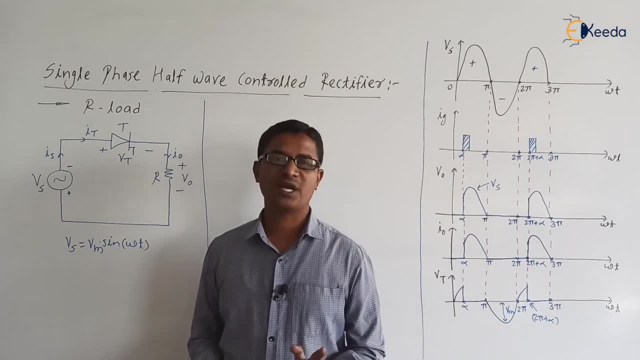 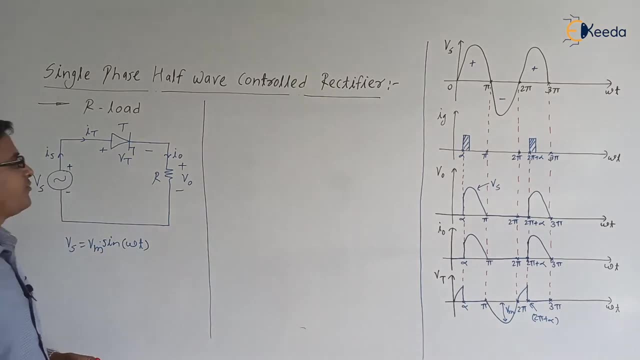 When Vs is negative, thyristor T will be in the reverse bias mode. So now let us discuss the circuit operation in each interval. So if you check for, omega T is equal to 0 to alpha. For omega T is equal to 0 to alpha. 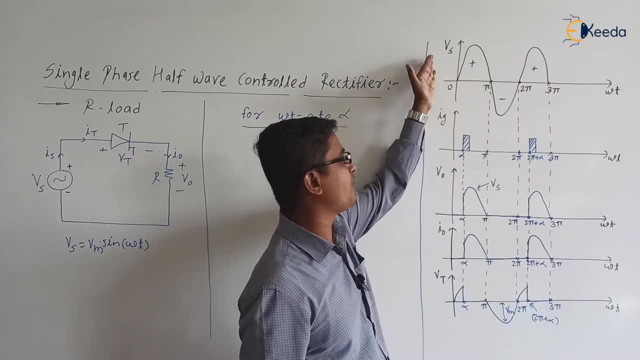 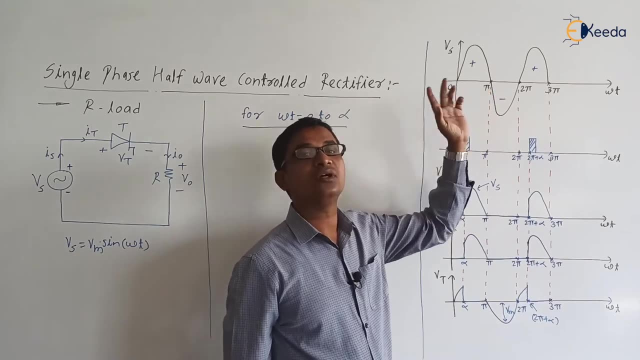 So if you check the waveforms here, it is a Vs waveform That is a sinusoidal voltage. So, as I said, when Vs is positive, thyristor will be in the forward bias mode. So if we want to turn on the thyristor with the help of gate signal, 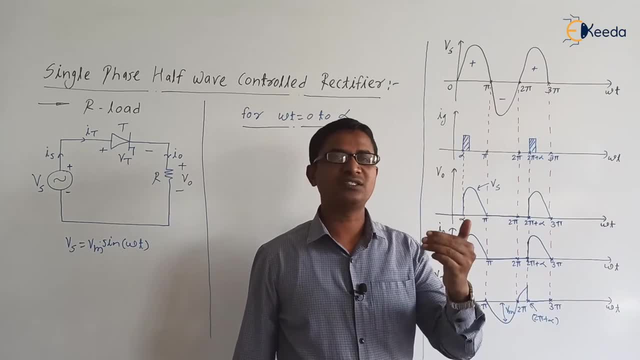 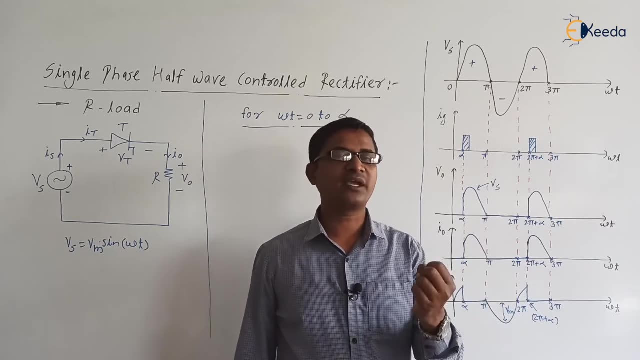 So first of all we need to check whether the thyristor is in the forward bias mode, If the thyristor is in the forward bias mode or not. If the thyristor is in the forward bias mode, then, and only then, we can turn it on by applying the gate signal. 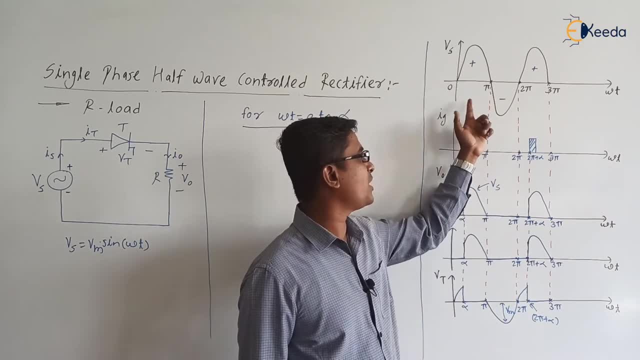 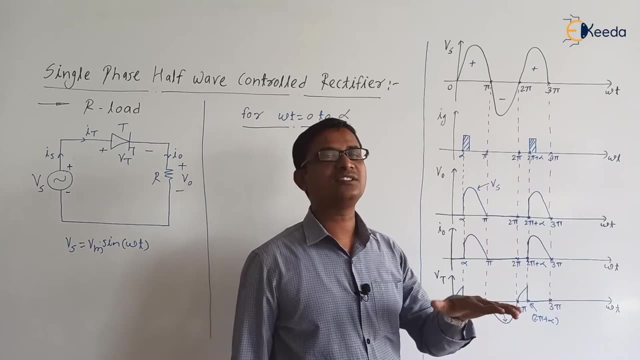 So as from omega T is equal to 0 to pi thyristor is in the forward bias mode. So that's why we have applied the gate signal. When Vs is negative, that is, from pi to 2 pi Thyristor is in the reverse bias mode. 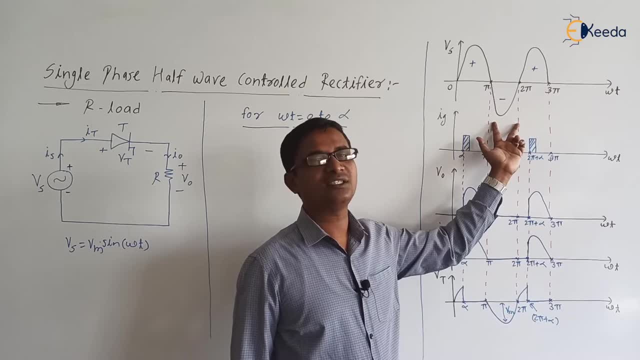 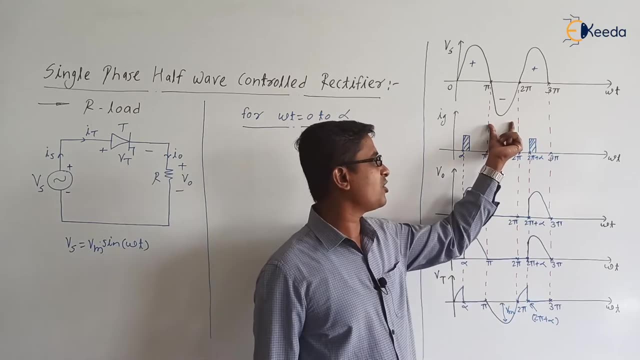 So during this interval thyristor will be in the reverse bias mode. So if the thyristor is in the reverse bias mode, If we apply the gate signal whether our thyristor will turn on? No. So during reverse biasing of the thyristor we have not applied the gate signal. 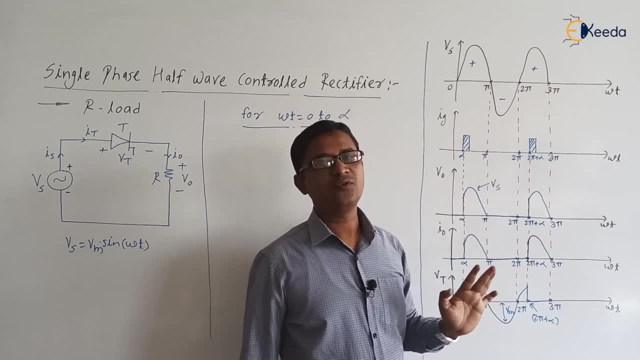 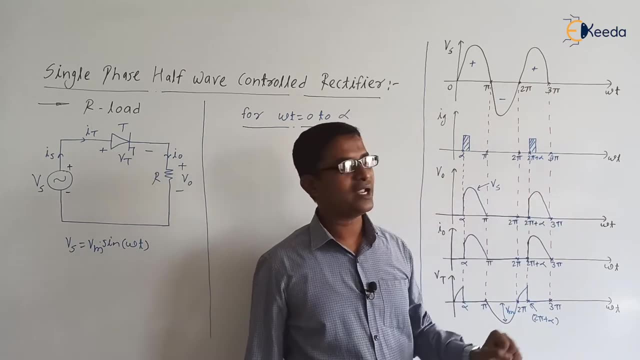 Next, from 2 pi to 3 pi, Vs is positive. Vs positive means thyristor is in the forward bias mode. So thyristor is in the forward bias mode. So we have applied the gate signal to the thyristor at 2 pi plus alpha. 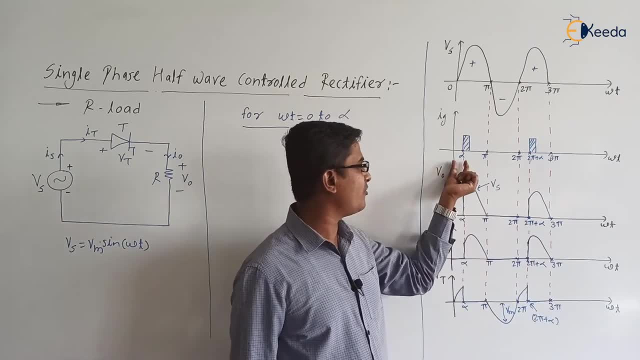 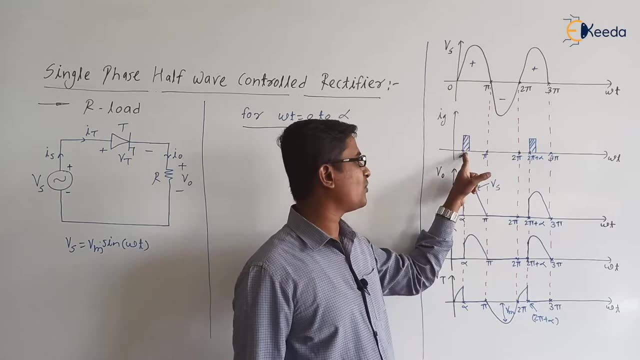 Alpha is the firing angle, So this angle is alpha. This is nothing but the firing angle of the thyristor. Firing is nothing but the triggering Means. at this instant we are applying the gate signal to the thyristor, So therefore our thyristor will turn on at omega. t is equal to alpha. 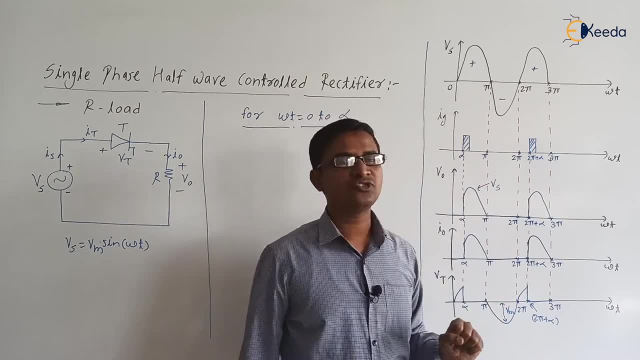 Because already it is in the forward bias mode. So when thyristor is in the forward bias mode, as we know, thyristor is a four layer, three junction device. Three junctions are J1, J2, J3.. 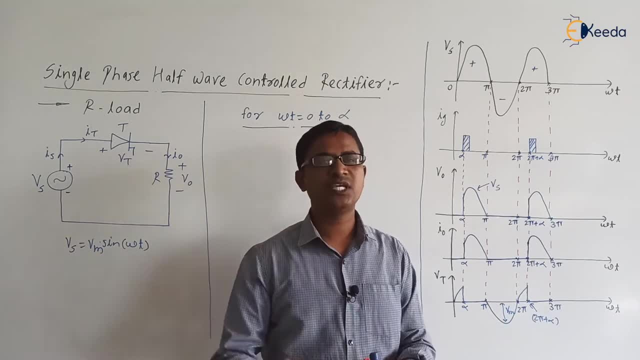 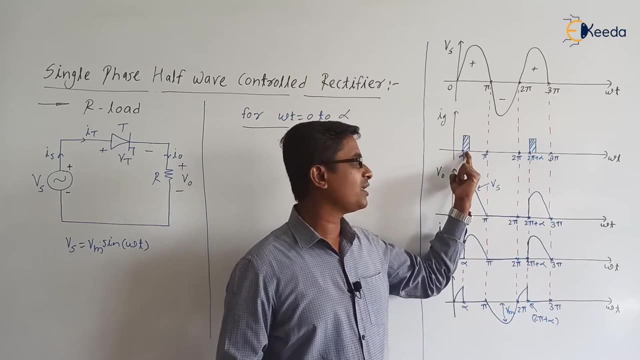 So J1, J3 are already in the forward bias mode. J2 is in a reverse bias mode. So in order to reduce the width of the deflation layer across junction J2, we are circulating the gate current at omega t is equal to alpha. 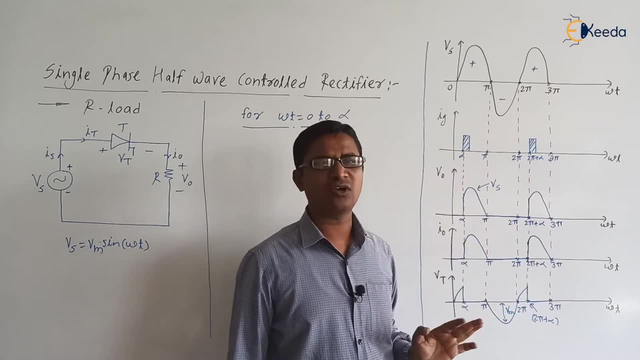 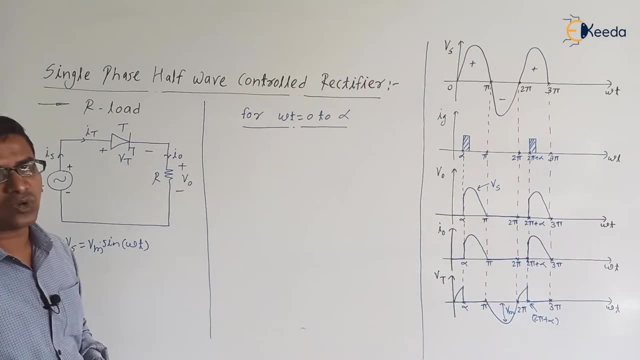 So after alpha, or at omega t is equal to alpha, Our thyristor will turn on. definitely So next. So if you check for omega t is equal to 0 to alpha, Now for omega t is equal to 0 to alpha. 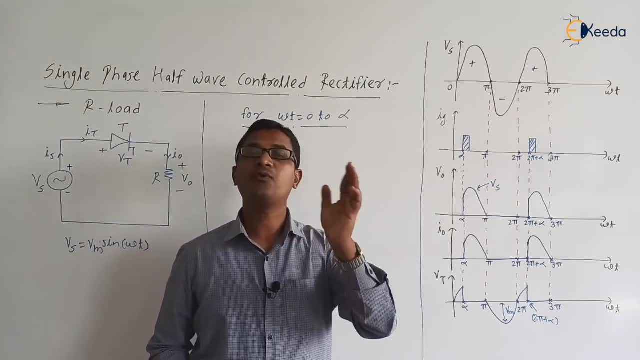 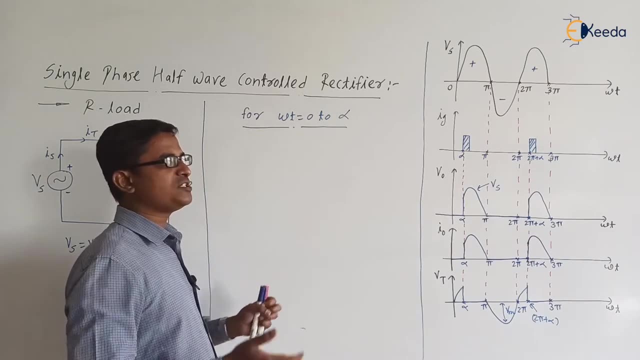 Whether we have applied the gate signal between 0 to alpha. No, We have applied the gate signal at alpha actually, So from omega t is equal to 0 to alpha. Or we can write: omega t is in between 0 and alpha. 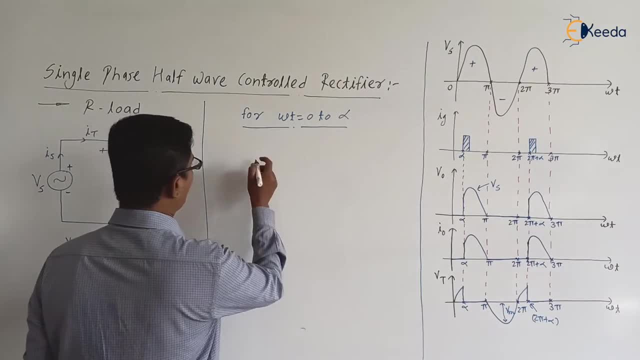 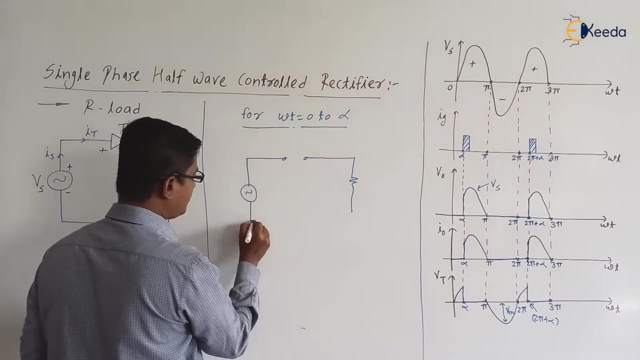 So yes, thyristor will be in the forward bias mode, But we have not applied the gate signal. Ok, So this is Ves volt, This is thyristor, This is Vt, This is It And this is Is. 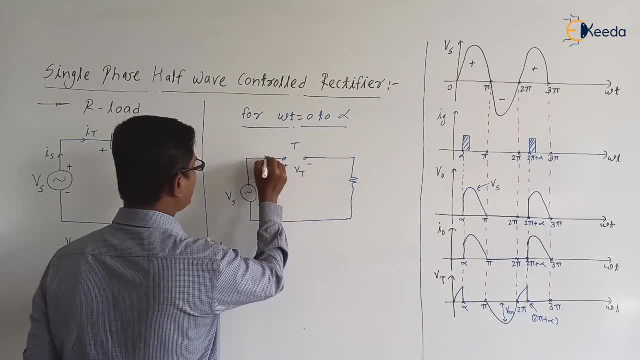 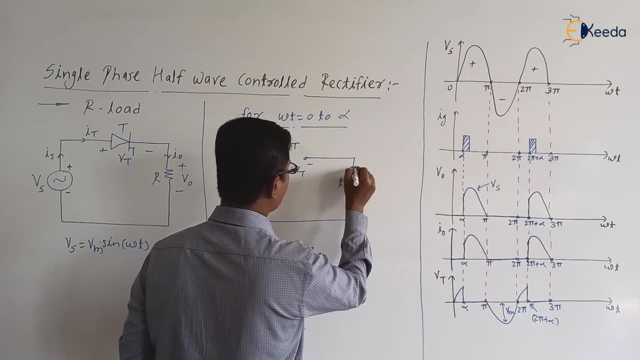 Supply current Is Purely resistive load. This voltage is V0.. This is current is I0.. Ok, So now, if you check, From omega, t is equal to 0 to alpha, Vs is positive, Vs is positive, But we have not applied the gate signal to the thyristor. 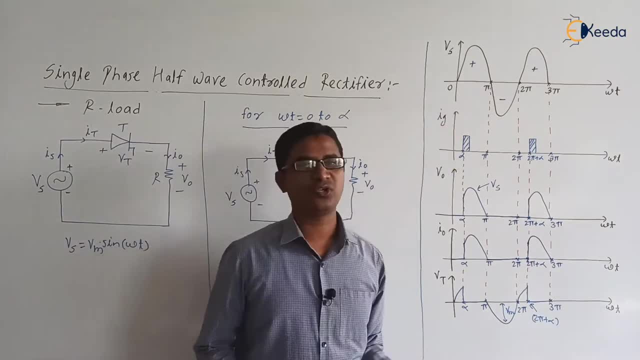 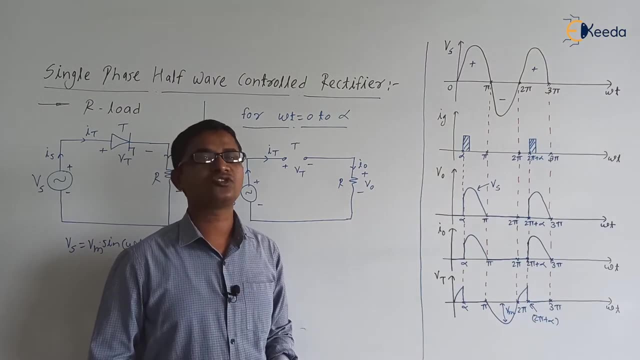 Ok, So for omega t is equal to 0 to alpha. It is positive. It is positive, But we have not applied the gate signal to the thyristor thyristor. okay, so we have not applied the gate signal thyristor. so what is the mode of operation? 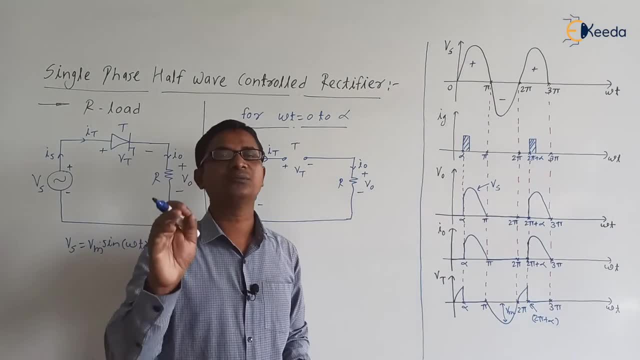 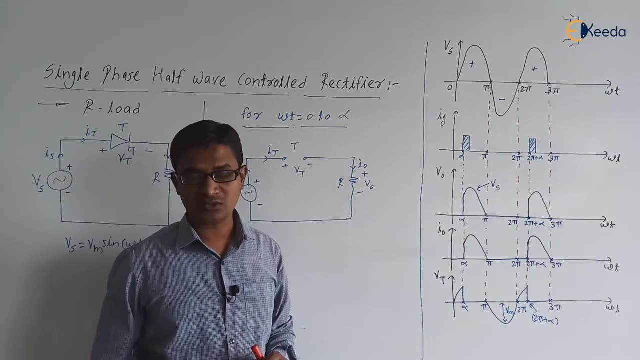 of thyristor. thyristor will be in the forward blocking mode. okay, recall the three modes of operation from the static vi characteristic of the scr? okay, which are those three modes? forward blocking mode, forward conduction mode and reverse blocking mode. okay, so here thyristor is. 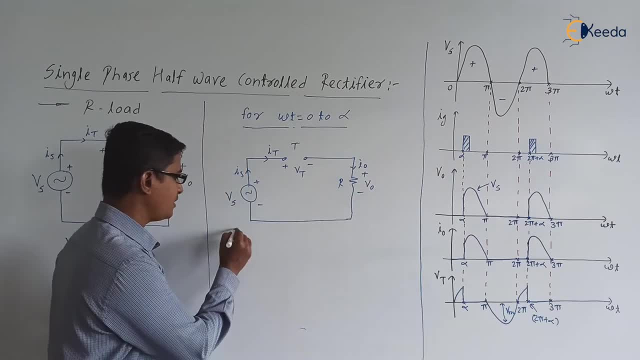 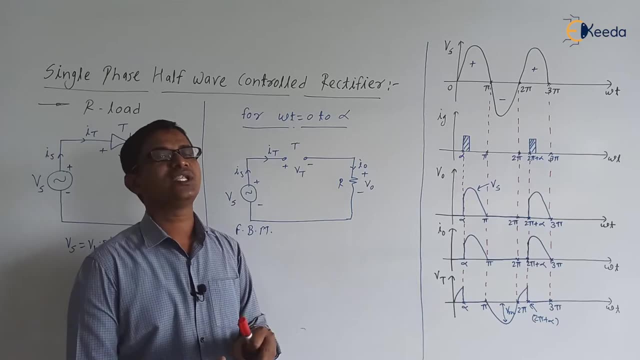 in the forward bias mode, but we have not applied the gate signal, so mode of operation will be forward blocking mode. right during forward blocking mode, thyristor voltage is high, current is very less, means thyristor will be acting as an open switch only. okay. so here thyristor will. 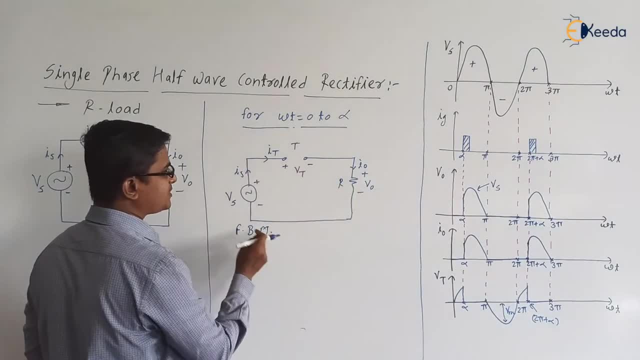 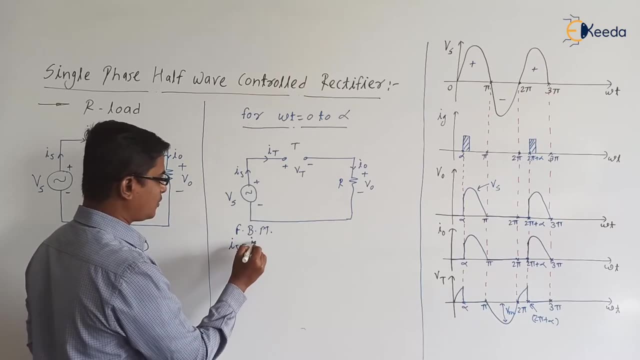 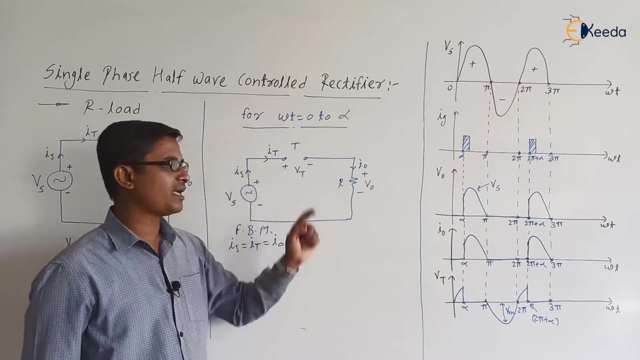 be in the off state. okay, so from 0 to all 5 thyristor is in the off state. yes, can we say that the current in the circuit is 0? definitely, so current in the circuit is 0, so we can write: is is equal to, it is equal to i0. is equal to what? 0 ampere? right, all the three currents? is it and i0? 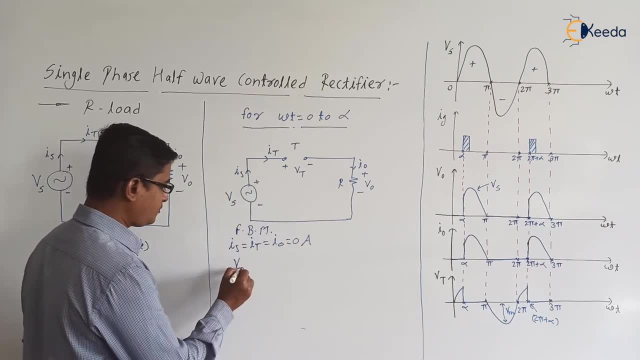 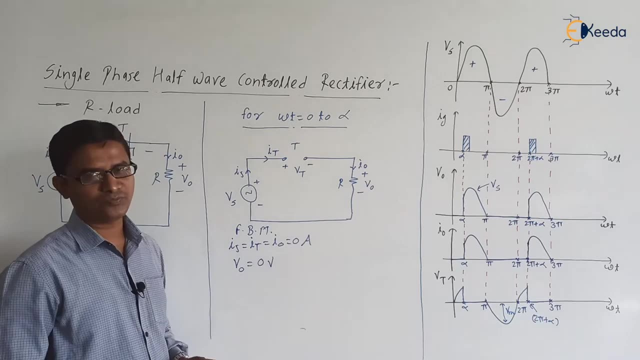 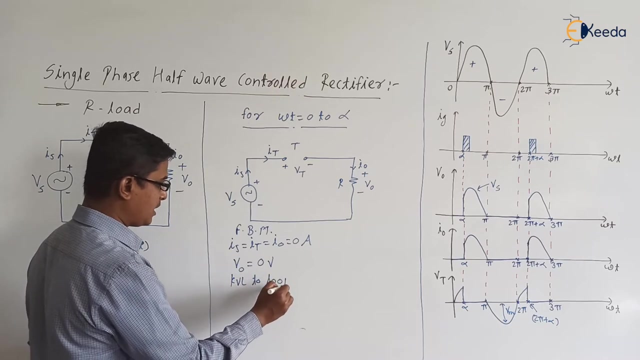 all are 0. okay, next, what is v0? according to Williams law, v0 is equal to i0 into R, right, so i0 is 0, so therefore v0 is also equal to 0. next, can we apply K VL to loop? yes, we can write K VL 2 loop. K VL 2 loop. so. 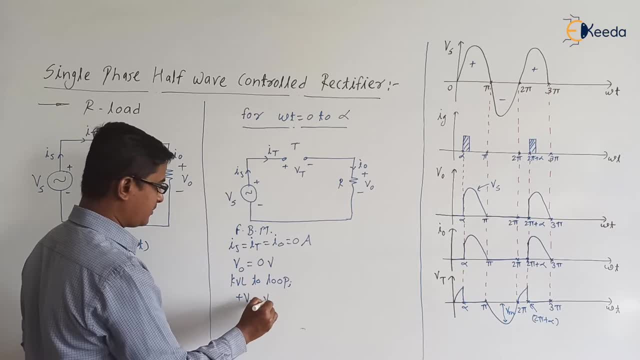 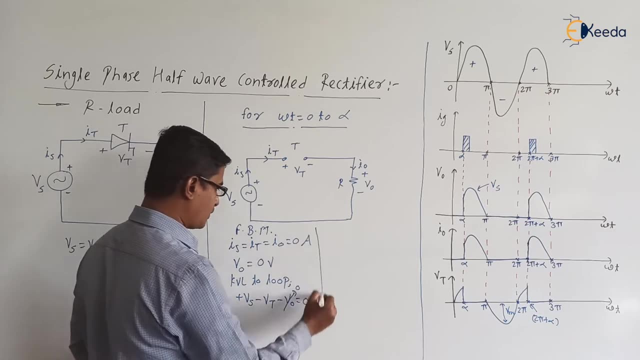 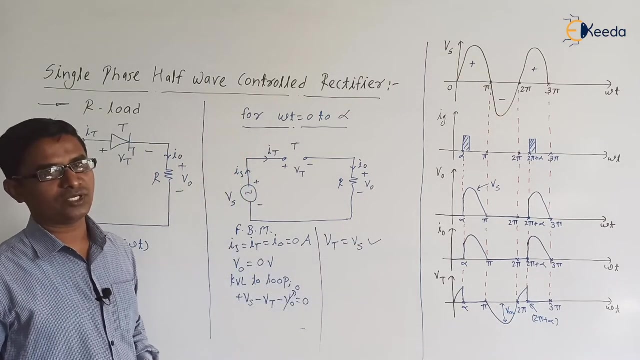 it is plus vs minus. vt minus v0 is equal to 0. okay, out of that, v0 is 0. so can we write it as ø is equal to vs? yes, we can write is equal to v? s. so thyristor voltage is same as that of the supply voltage. okay, so if you check, 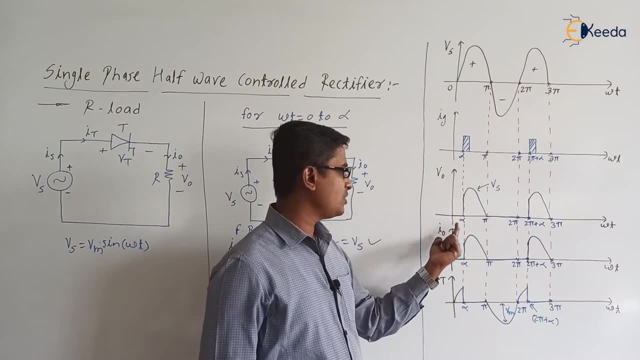 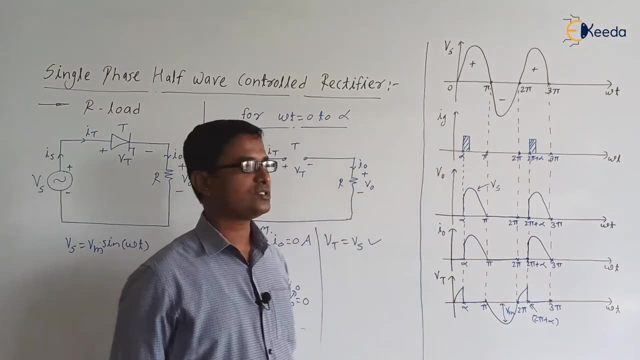 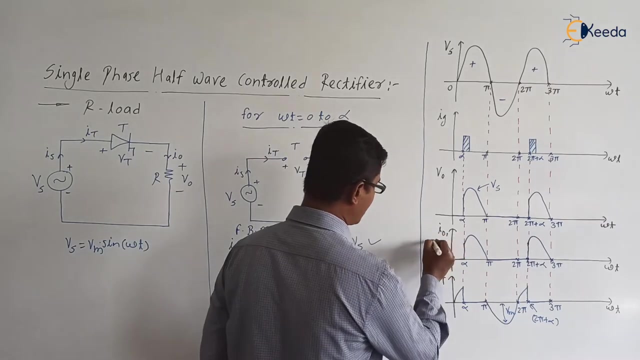 from omega. t is equal to zero to alpha. okay, so v? zero is zero, i zero is zero, right? i zero zero. v zero, zero, right. what is v? t? v? t is same as that of the supply voltage. v? t is same as that of the supply voltage. okay, right again, i zero and i? t and i s- all are same. so here we can add the terms i. 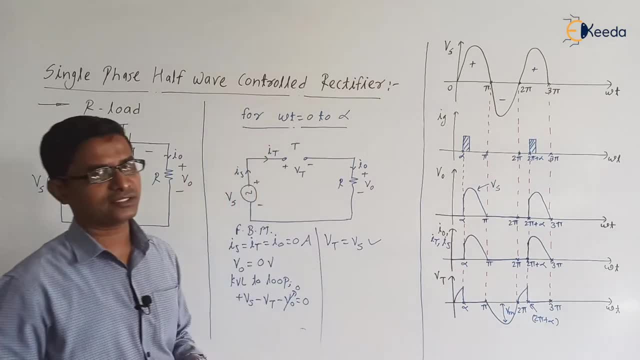 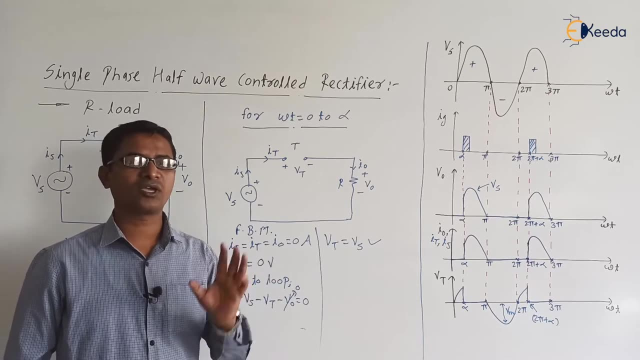 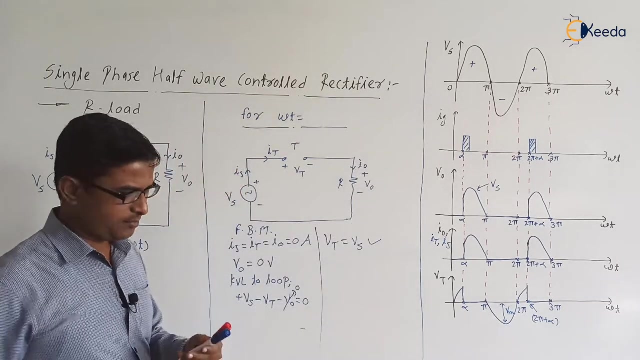 zero, i t and i s okay. i, zero, i t, i s. all are same right. zero to alpha. next. is this clear? so during zero to alpha, thyristor will be in the forward blocking mode, okay. next let us discuss. for omega t is in between alpha to pi. for omega t is in between alpha to pi, alpha to pi- okay, so during. 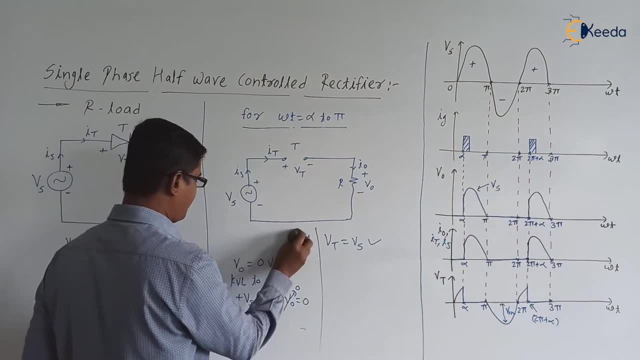 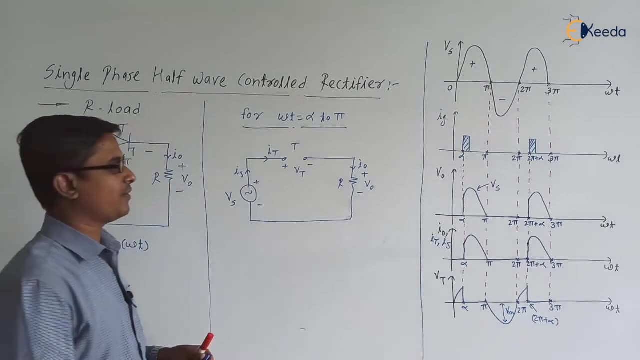 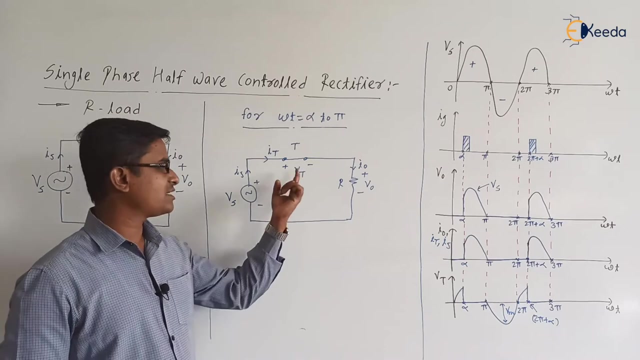 alpha to pi. right, so at omega, t is equal to alpha. we are applying the gate signal to the thyristor. okay, right, so our thyristor will turn on at alpha. right, so at alpha, our thyristor will turn on. okay, so thyristor will act as a short circuit. okay, so, once thyristor acts as a short circuit, 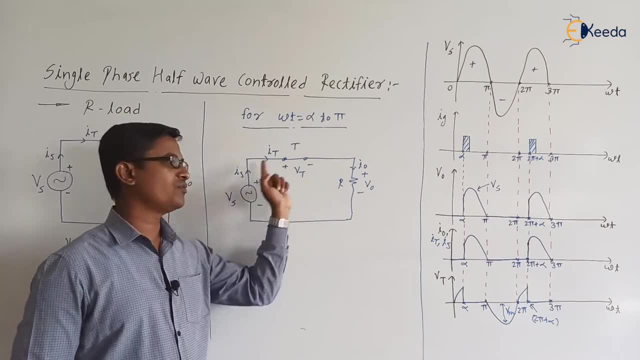 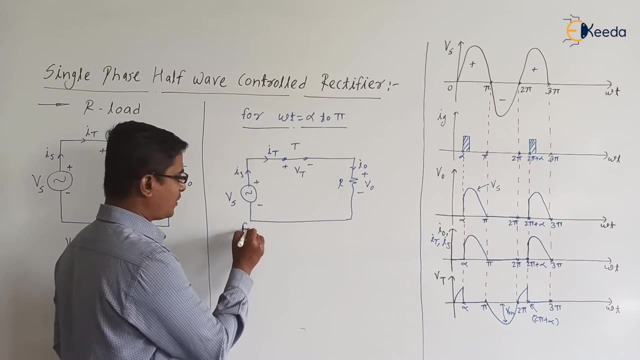 current will be flowing from v s thyristor load and again back to the v s, so in this loop the current will be flowing, okay. so what is the v? t or, first of all, what is the mode of operation of thyristor? it is a forward conduction mode. are you getting the point zero to alpha? it was a. 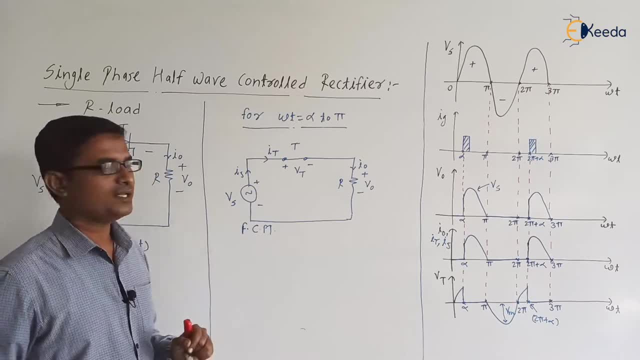 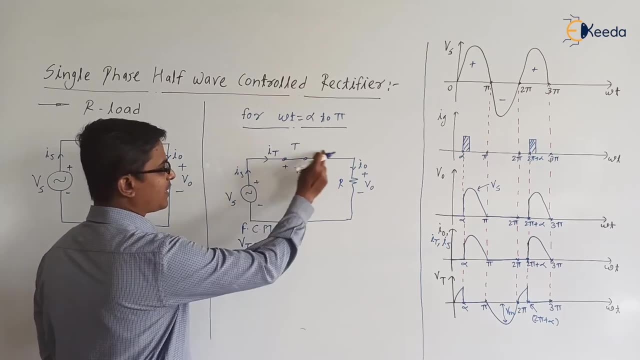 forward blocking mode. now it is a forward conduction mode. okay, so next, what is the v t? yes, thyristor is acting as a short circuit, so v? t is equal to zero volt. right next, can we apply kvl to the loop? yes, kvl to loop is plus v s, minus v t, minus v. zero is equal. 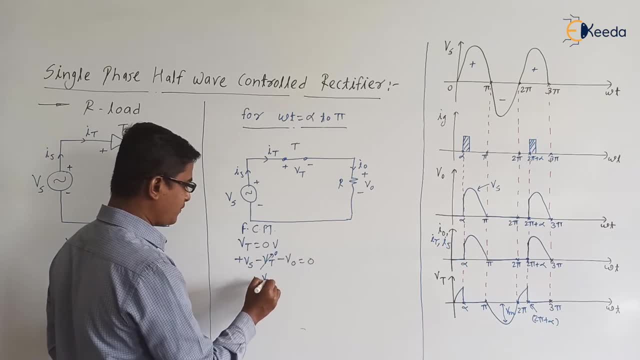 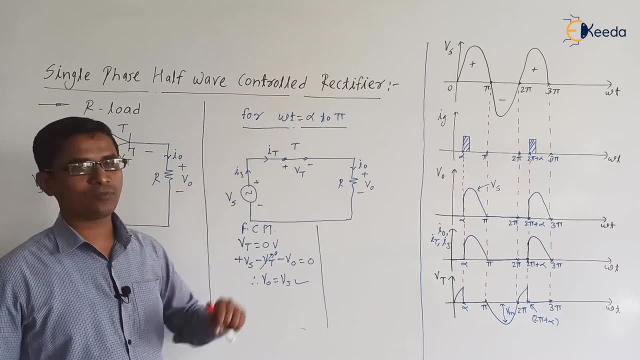 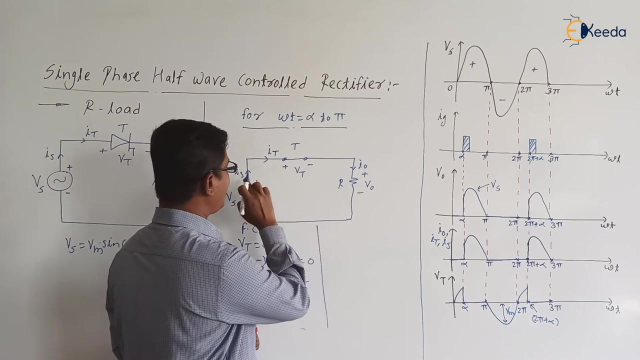 to zero. out of that v t is zero, so we can write it as a: v zero is equal to v s right. so output voltage is same as that of the supply voltage from alpha to pi. okay next, so v zero is same as that of the vs right. next, what is i0? as we know, i0, it and is all are same because we are having only one loop. 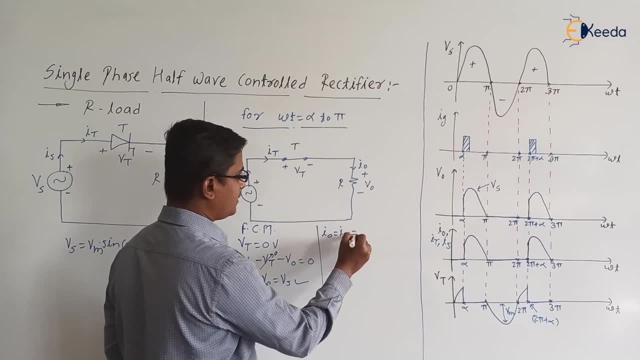 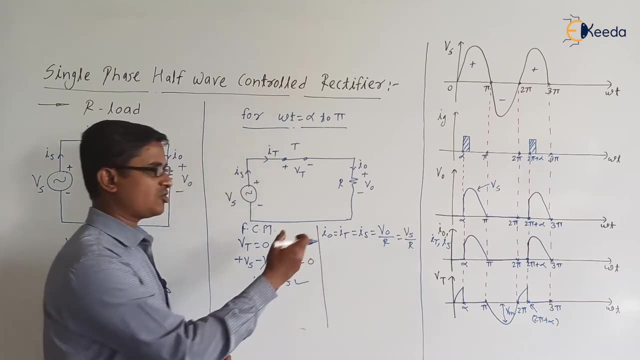 okay, so i0 is equal to, it is equal to, is is equal to what: v0 by r, which is equal to vs by r, because v0 is same as that of the vs, so it is a vs by r. are you getting the point, okay? so if you check, 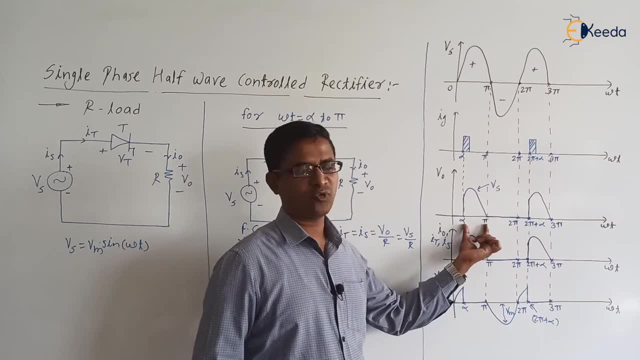 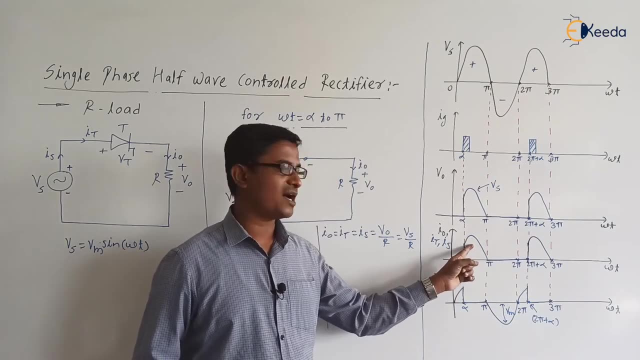 for omega t is in between alpha to pi. for omega t is equal to alpha to pi. what is v0? v0 is same as that of the supply voltage i0. yes, it is a vs by r. so it is a vs by r means what v0 i0 will be. 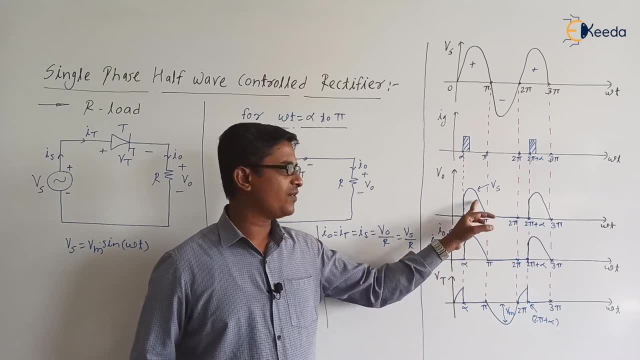 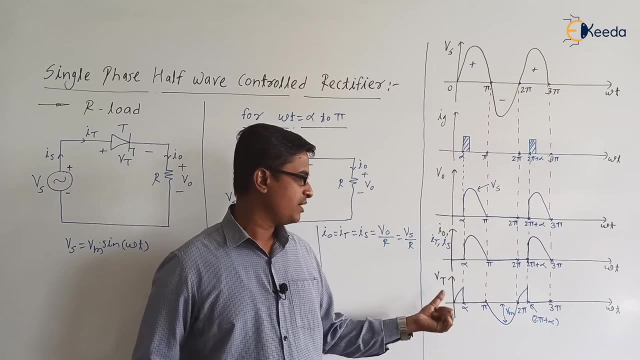 in phase with v0. are you getting the point? i0 will be in phase with v0, right? because it is a v0 is vs and i0 is vs by r. okay, so it will be in phase with v0. next, what is vt? vt is zero. from alpha to. 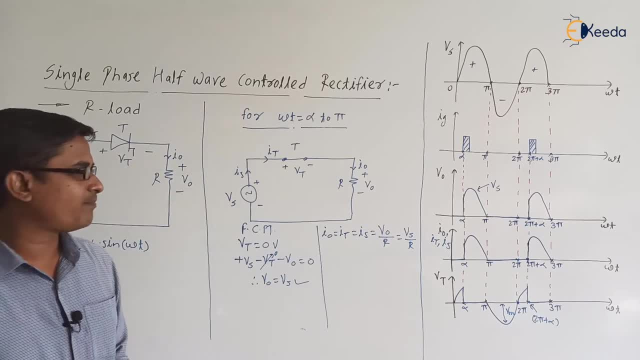 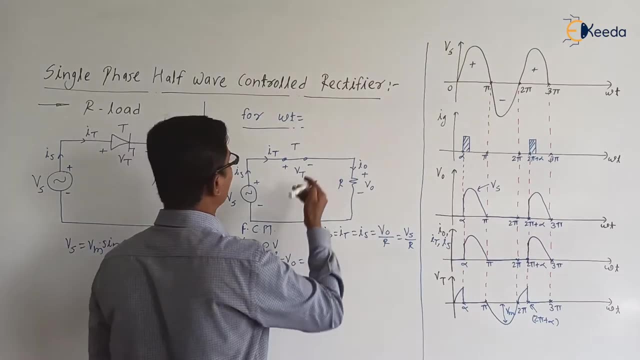 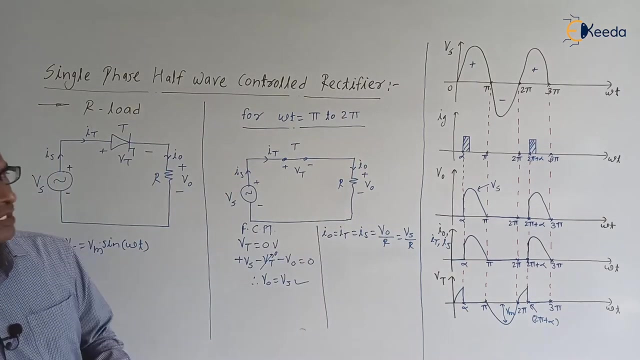 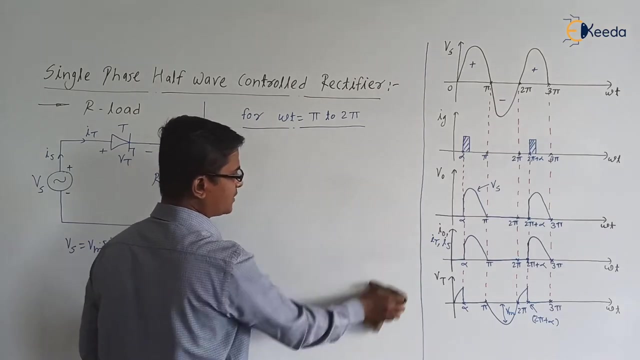 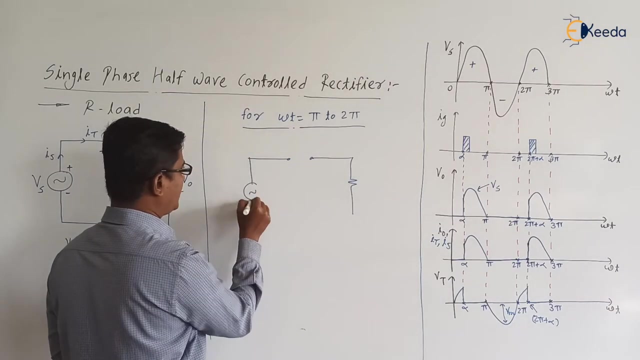 pi. okay, next after pi. after pi: yes, let us discuss what will happen. from alpha to sorry, from pi to 2 pi, for omega t is equal to pi to 2 pi. let us discuss what will happen. okay, so if you check after pi, the supply voltage is reversed. right, supply voltage is reversed. so if the supply voltage is reversed, 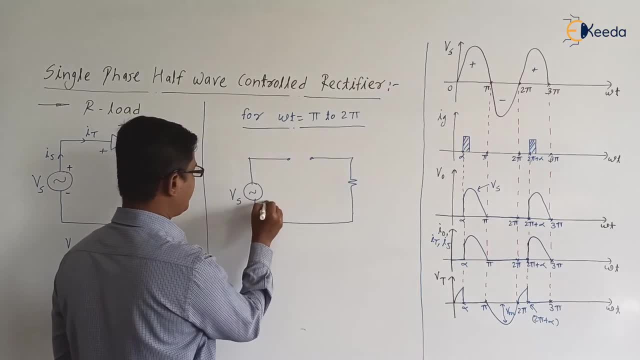 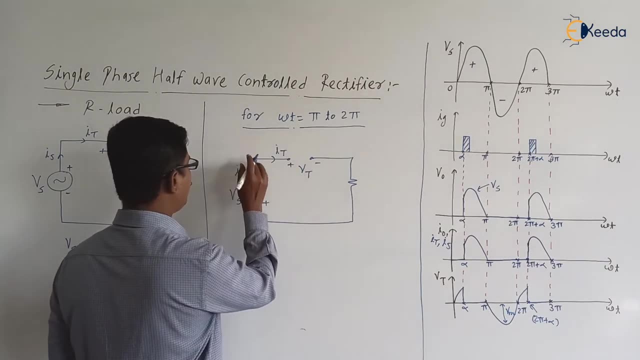 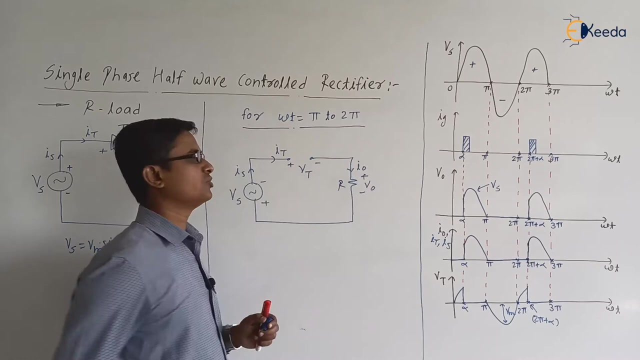 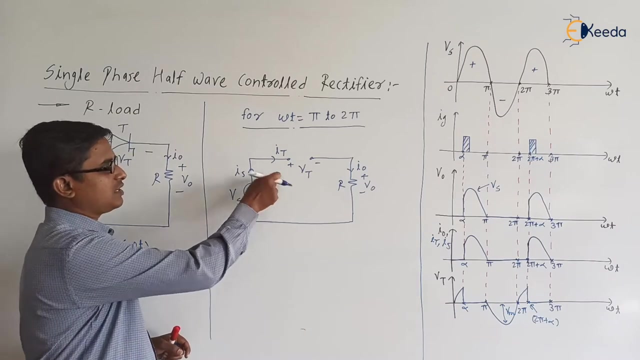 the reverse voltage vs. this is vt, this is it, this is is r, v0 and this is i0. okay, so after pi the supply voltage is negative, right after pi the supply voltage is negative. supply voltage is negative means we have, yes, reverse the polarities of the supply voltage vs. okay, so minus here and plus here. okay, so this is the. 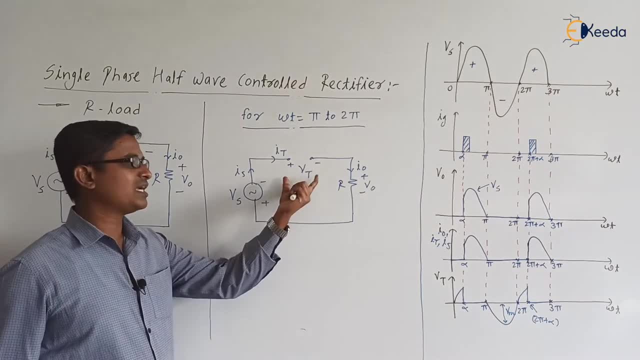 lowest potential point. this is the highest potential point, okay. so definitely, our thyristor will be in the reverse bias mode, okay. so if you check, thyristor is in the reverse bias mode, okay. so, if you check, thyristor is in the reverse bias mode, okay. so if you check the highest 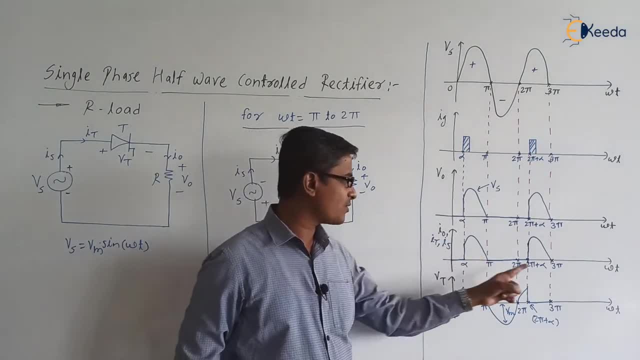 the highest and following the direction in thyristor is in the reverse bi t instant. and if you check the published形, a or i0 wave form at omega is equal to pi, at amhal force, bi with a function of מש and at omega is equal touke in order to be able to. 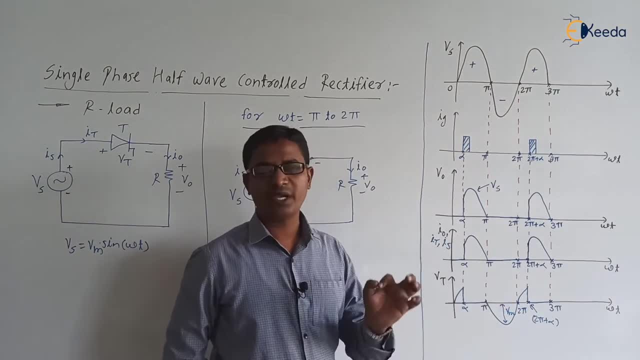 equal to the i plane constant spin somas. phi current flowing through theline becomes equal to 0 at algorithm. t is equal to phi current flowing. cool thyristor. interesting event at omega Maritimo of this new indian you know bad. so current flowing fully. 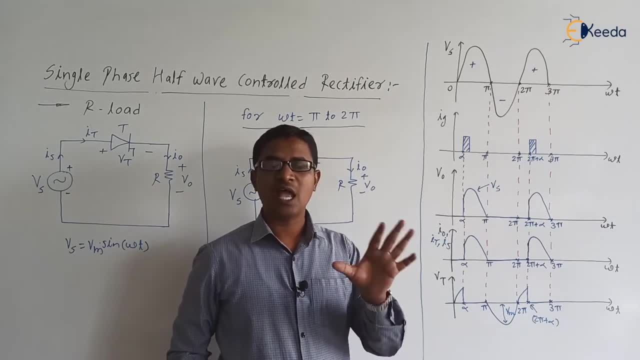 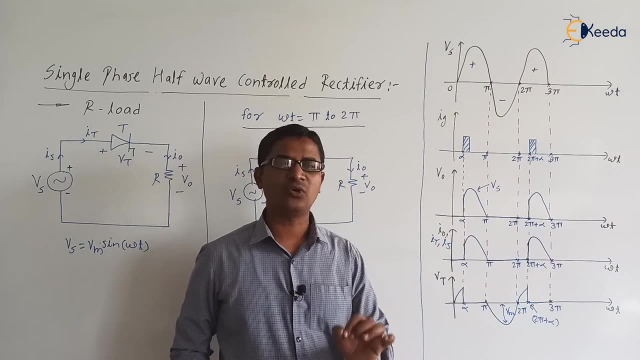 that id of the flops equal to zero. the meaning is: is like a could not of the pressure крит r Orgod ir nicely okay. so when these zero value of and current is less than the volt of current value, definite lyatory Emp bu jà. 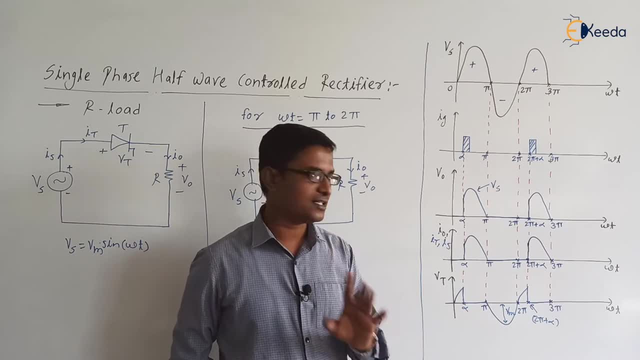 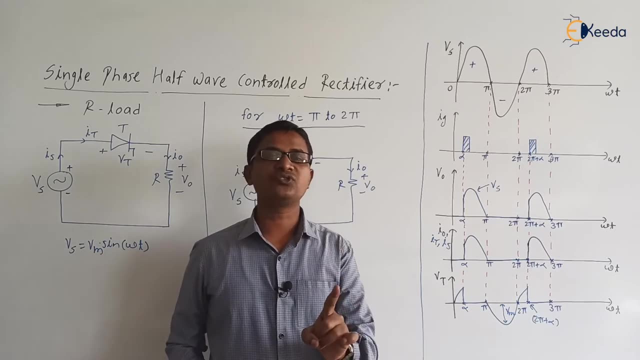 we say that the first condition for commutation of thyristor has reached at omega t is equal to pi. yes, recall the procedure for commutation of thyristor. first step. first of all, we need to reduce the anode current value less than the holding current value right which has reached. 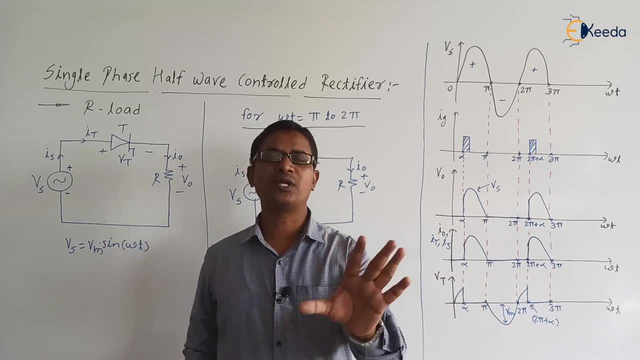 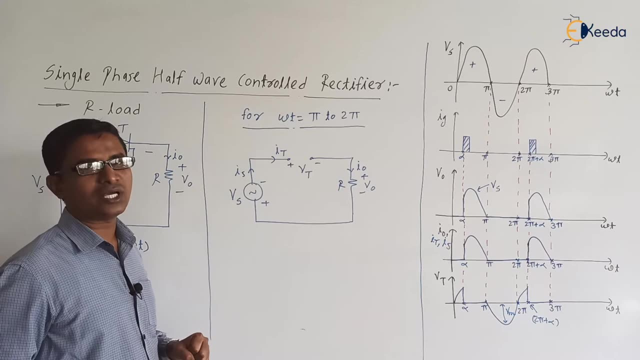 at omega t is equal to pi. after that, we need to maintain the reverse voltage across the thyristor. okay, so if you check the circuit, if you check the circuit right due to the nature of the supply voltage, due to the nature of the supply voltage after omega t is equal to pi, right, due to the 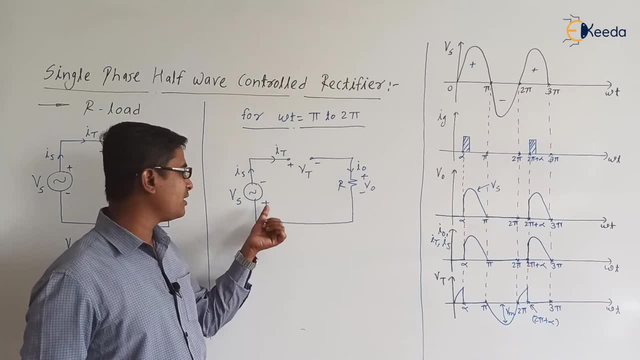 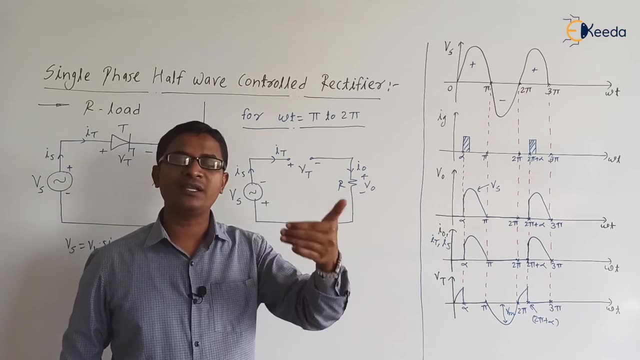 nature of the supply voltage. after omega t is equal to phi, automatically the reverse voltage will be maintained across the thyristor. are you getting the point okay? so how we are maintaining the reverse voltage across the thyristor? yes, it is due to the nature of the supply voltage, so 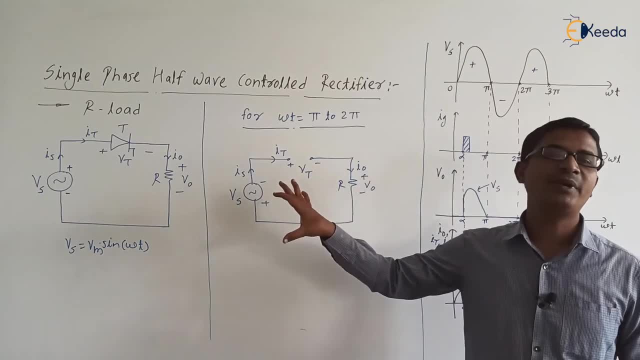 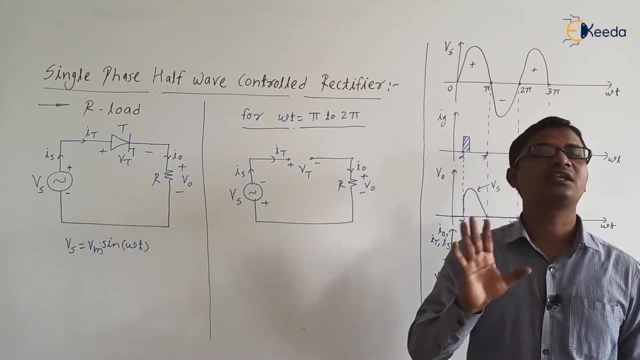 please be careful here. we have not added external elements right for successful turn off of the thyristor right. it is due to the nature of the supply voltage the thyristor is turning off or reverse, voltage is maintained across the thyristor. okay, so that's why it is known as the natural 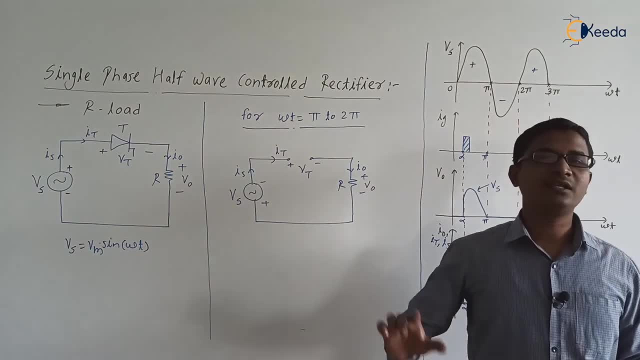 commutation. so in this type, in this type, as i said, in the rectifier circuitry, the input is ac, right, and when the input is ac, yes, the type of the commutation of the thyristor, yes, it will be the natural commutation right. so here, if you check at, omega, t is equal to phi, the current. 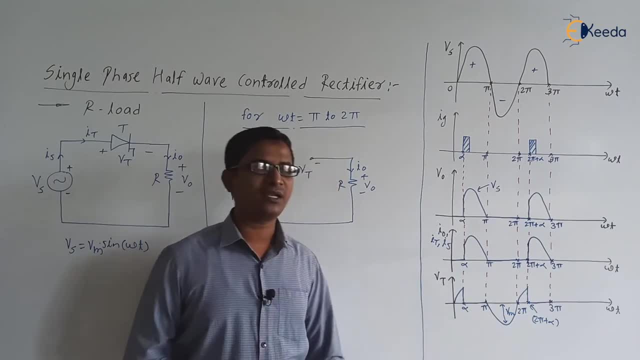 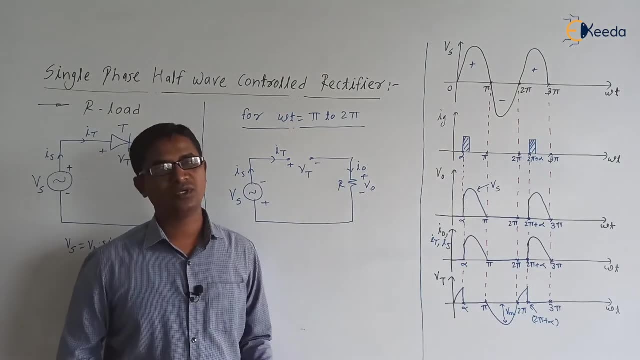 flowing through thyristor becomes zero and after that the reverse voltage will be maintained across the thyristor. this is due to, yes, reversal of the supply voltage right, reversal of the supply voltage right. so here at omega, t is equal to pi. our thyristor will. 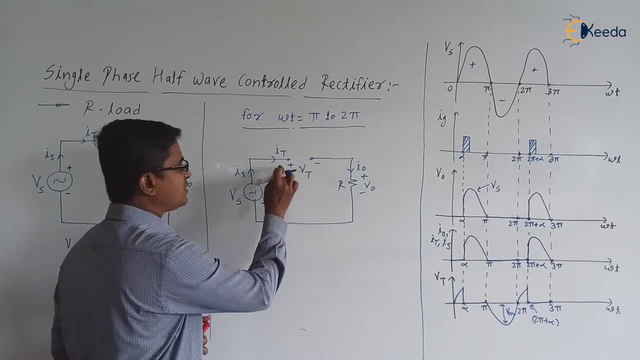 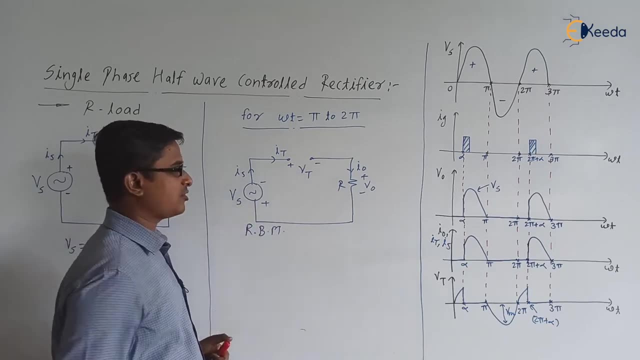 successfully turn off. okay, so from pi to 2 pi the thyristor will be in the reverse bias mode. okay, so mode of operation: it is a reverse blocking mode. mode of operation of thyristor: it is a reverse blocking mode, right, so thyristor will be acting as a open circuit, right? so now, in this case, if you, 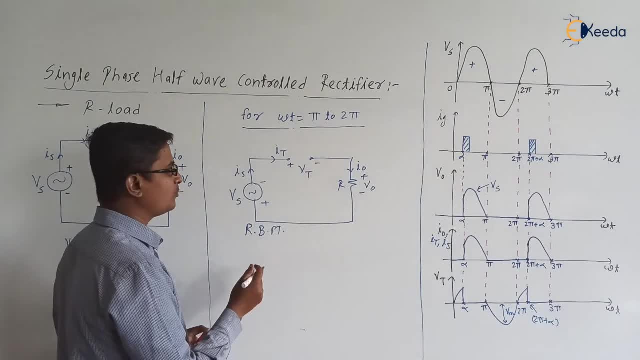 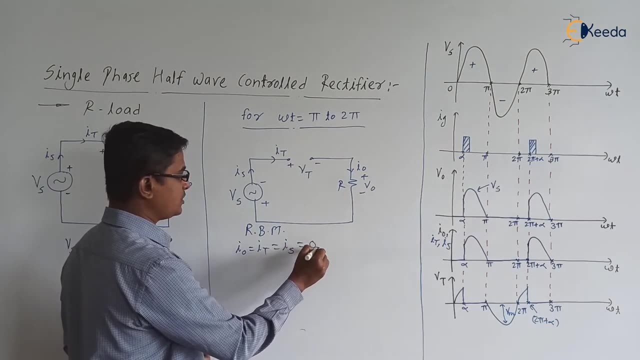 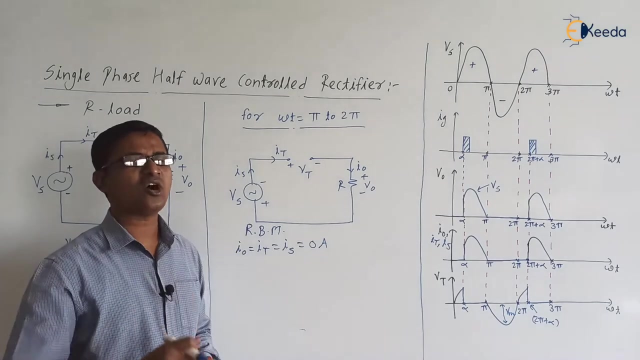 check thyristor is acting as an open switch, so what is the current in the loop? it will be zero. okay, so we can write it as i0 is equal to, it is equal to, is is equal to zero ampere, right? so i0 it is. all are zero, right from pi to 2 pi. our thyristor is in the opposite, so due to that, the 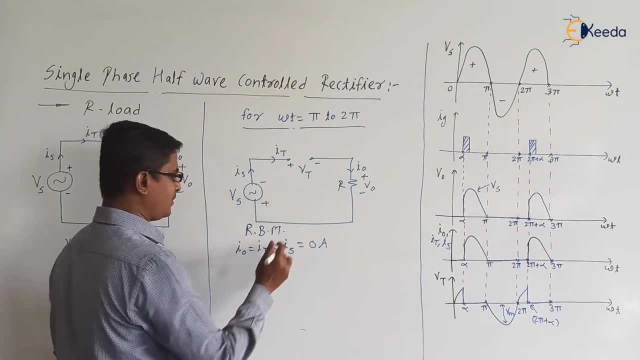 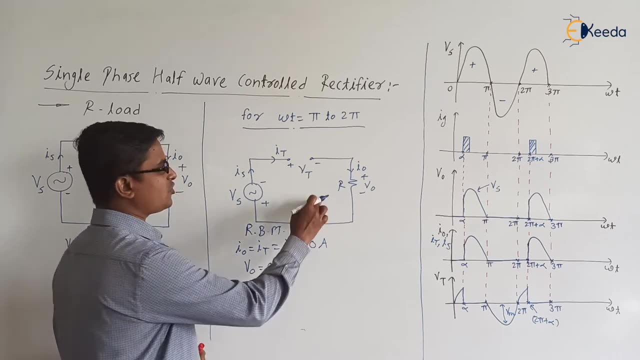 current will be zero next. so if the current is zero, what is the v0? v0 is equal to i0 into r according to the ohms law. so v0 is equal to zero volt right next. if v0 is zero volt, what is the vt? 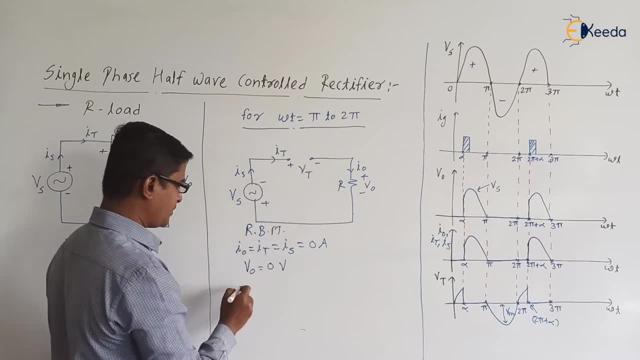 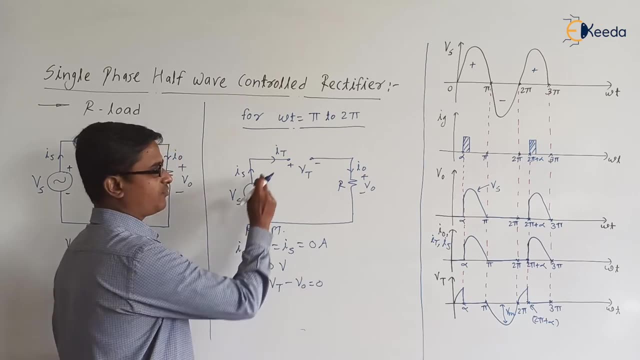 yes, we can apply the kvl and we can find vt. okay, so it is a. v0 is equal to i0 into r according to the ohms law, so v0 is equal to 0 volt, right next, if v0 is minus vs minus vt minus v0 is equal to zero, right? this is the kvl equation for this loop. 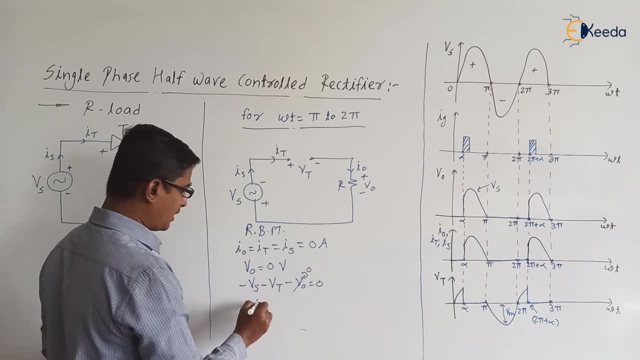 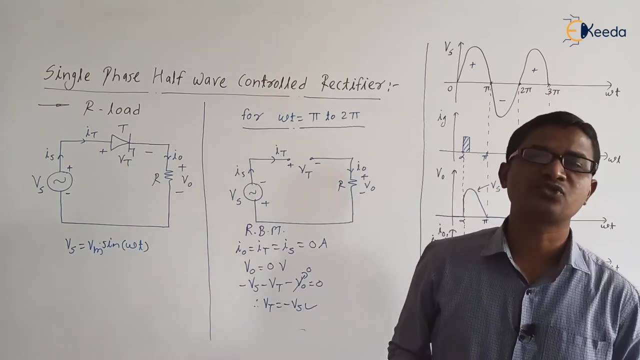 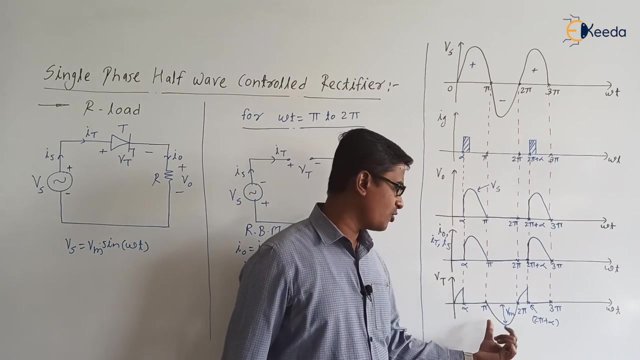 okay, out of this, v0 is zero, right, so we can write: vt is equal to minus vs. okay, so voltage across thyristor: voltage across thyristor will be the reverse voltage. right voltage across thyristor will be the reverse voltage. so if you check after or after, omega t is equal to pi or for. 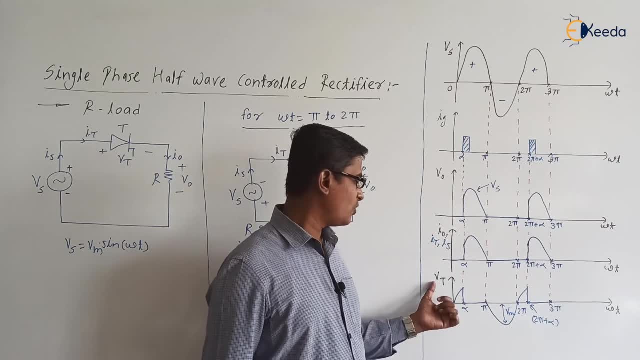 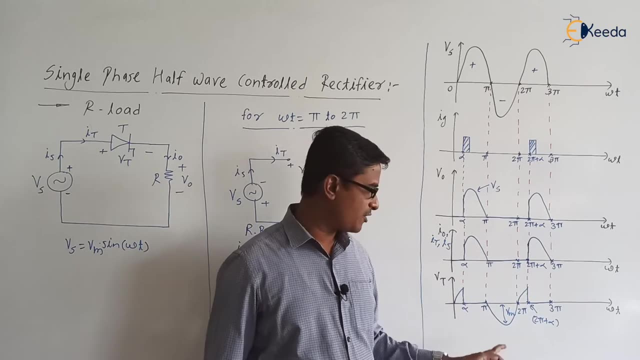 omega t is in between zero to two pi. yes, what is happening? the voltage across thyristor will be the minus vs right, so it is a negative voltage, but the magnitude will be same as that of the supply voltage that will be appearing across the thyristor. that will be 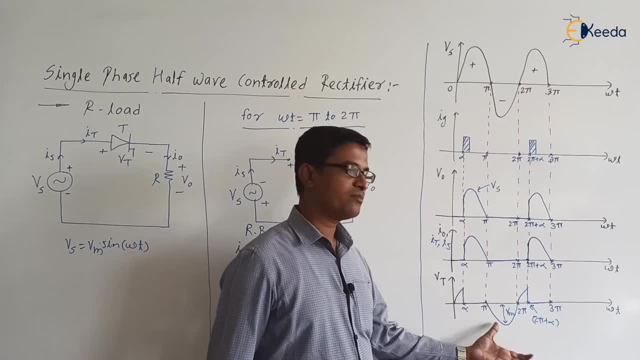 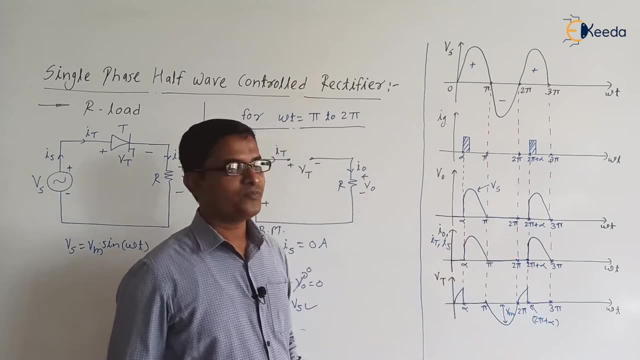 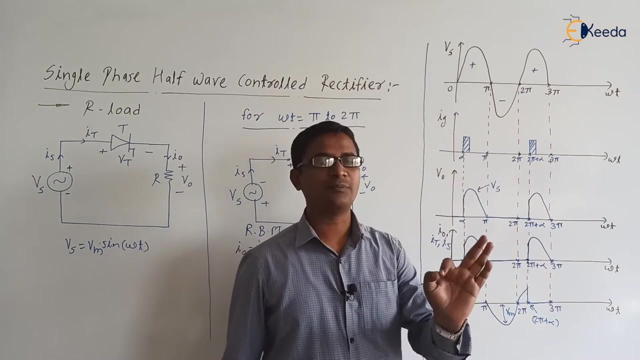 appearing across the thyristor. right, so from pi to two pi, vt is minus vs i0, it is is equal to zero, v0 is zero. are you getting the point? okay, so after 2 pi, what will happen? yes, whatever the waveform is here- 0 to 2 pi- one cycle of the supply is completing, right, so after 2 pi, second cycle will start. okay, 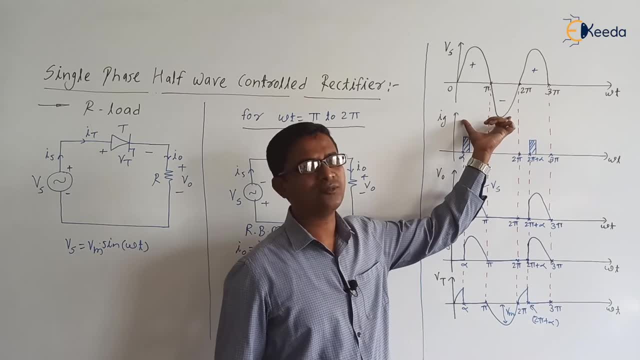 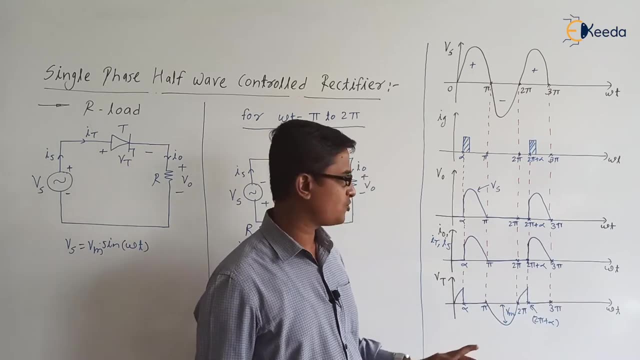 so whatever the waveform we are having in the output- right from 0 to 2 pi- the same will repeat from 2 pi to 4 pi. right, the same will repeat from 2 pi to 4 pi. are you getting the point? okay? so for: 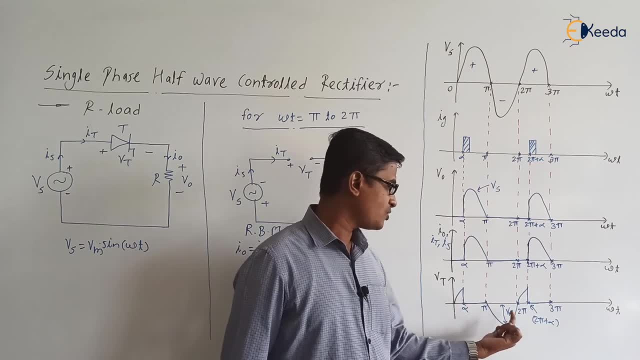 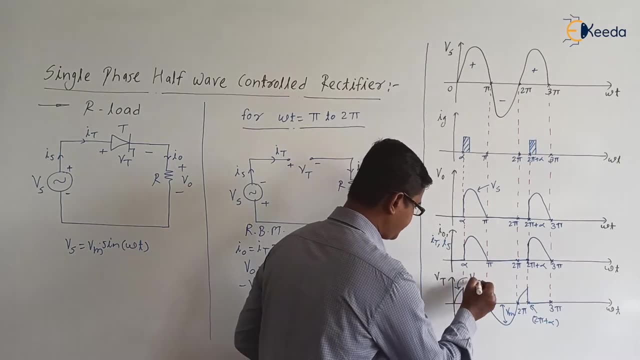 2 v vt. also right from 0 to alpha, it is a vs. so therefore, 2 pi to 2 pi plus alpha, it will be vs. only right, are you getting the point? so this is a vs, this is also vs, this is also vs. is this clear? 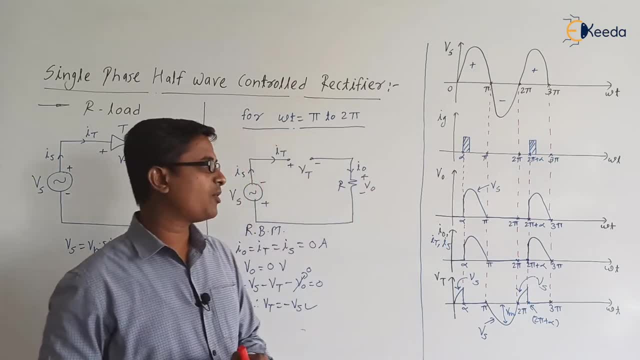 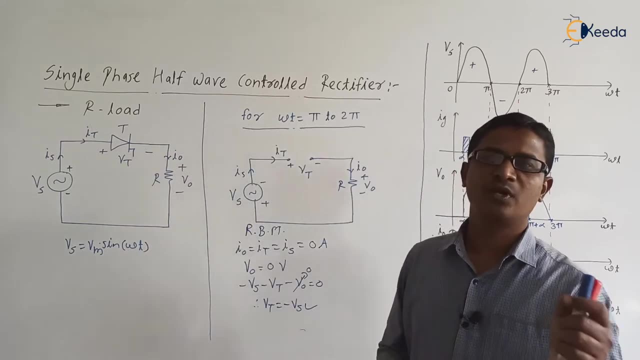 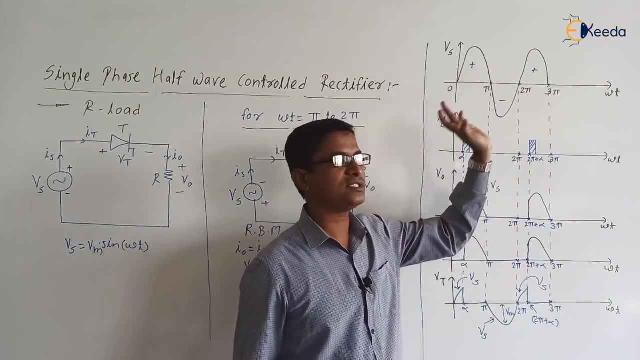 are you getting the point? okay, so this is about the circuit operation of single phase half wave control rectifier with purely resistive load. okay, so if you check the output voltage waveform here, v0. here supply voltage is positive and negative means it is a sinusoidal, it is a ac voltage. okay, v0 here we. 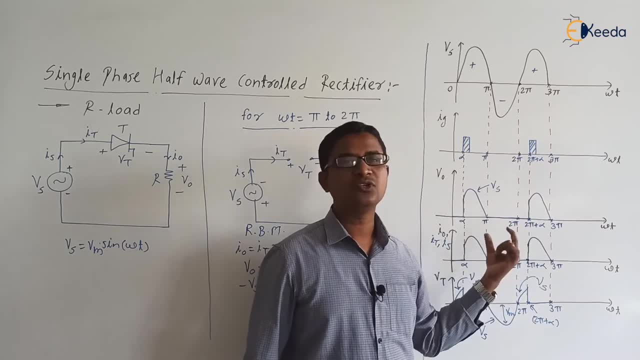 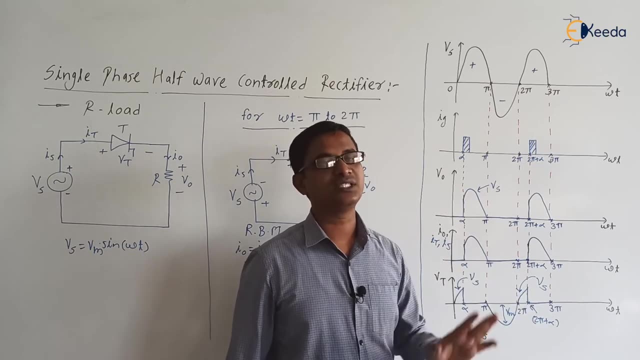 have the zero value, positive value. zero value, positive value. okay, so it is a dc. okay, output voltage is having only single polarity. that is a positive. okay, positive value. so that's why it is a single. okay, wszyscy 알고. commissioner say i am getting one flight per second, okay, but it is a. 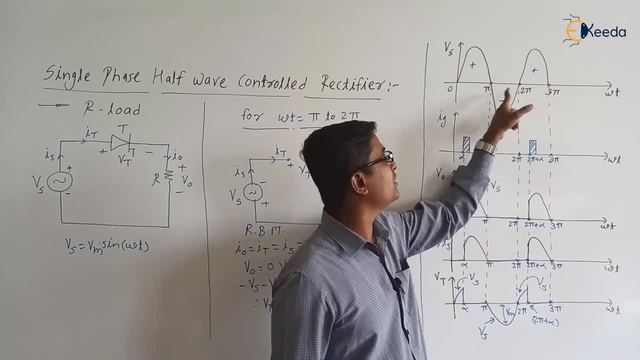 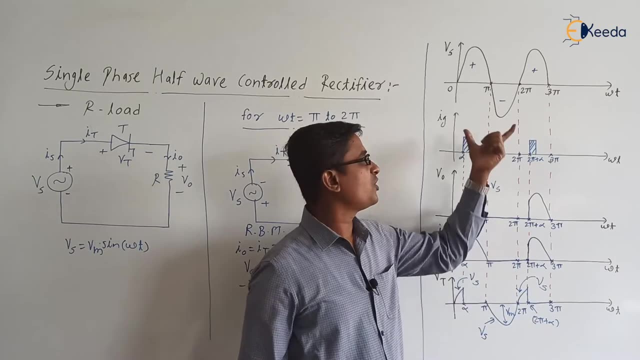 flat dc. no, it is a pulsating dc. output is a pulsating dc. next, if you check, corresponding to one input cycle, that is from 0 to 2 pi corresponding to one input cycle in the output, we are getting only one pulse corresponding to one input cycle. in the output we are getting 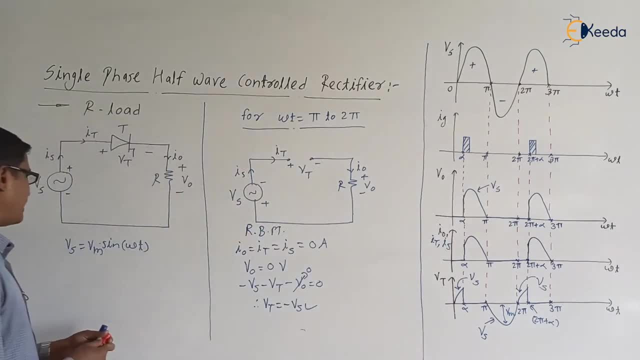 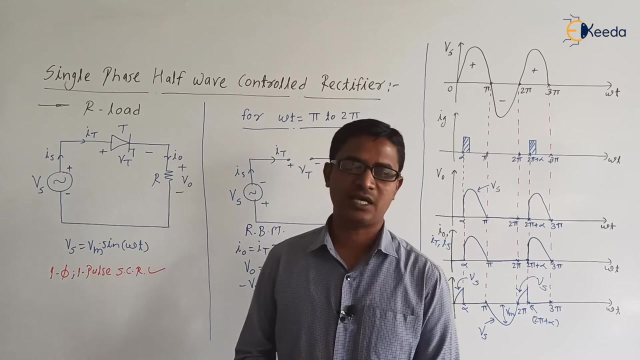 only one pulse. that's why it is known as a single phase single pulse rectifier. okay, it is also known single phase, yes. single pulse, yes, cr. some of the times they have asked the question like: in a single phase, single pulse, scr. so if they use the wording single phase, single pulse, scr or 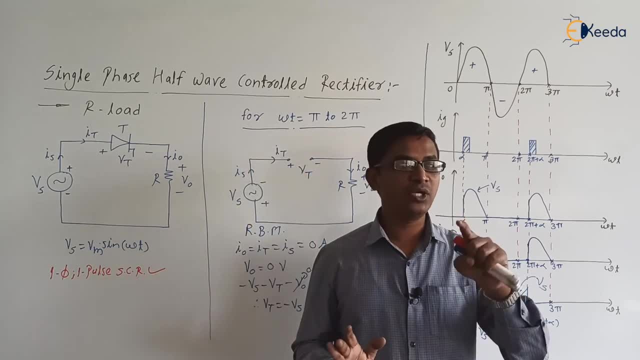 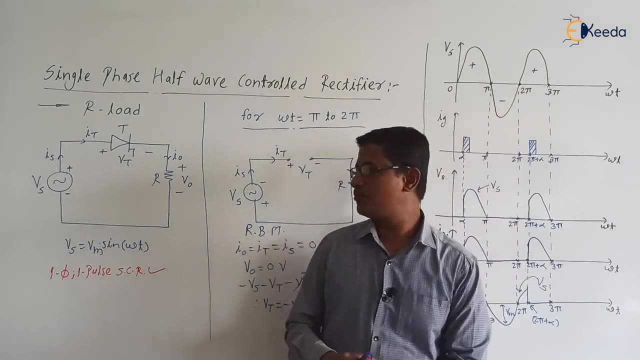 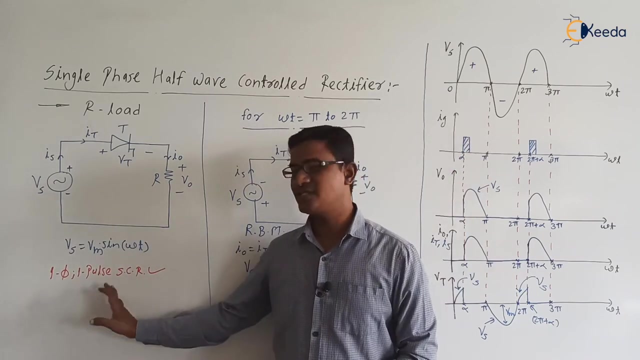 single phase, single pulse rectifier, then you need to understand. it is a half wave rectifier, are you getting the point? because corresponding to one input cycle, single phase, means what? corresponding to one input cycle, right, single phase we are having. okay, corresponding to one input cycle, in the output we are getting only one pulse. that's why it is a single phase, single pulse. 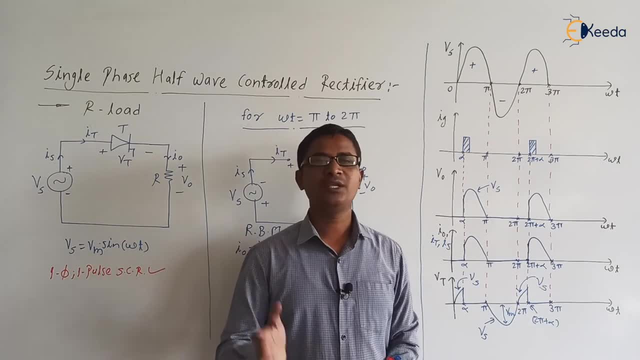 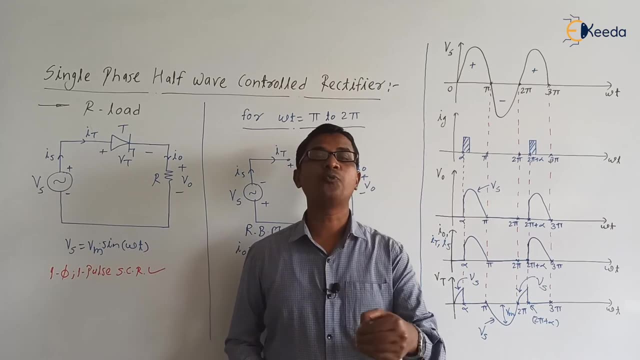 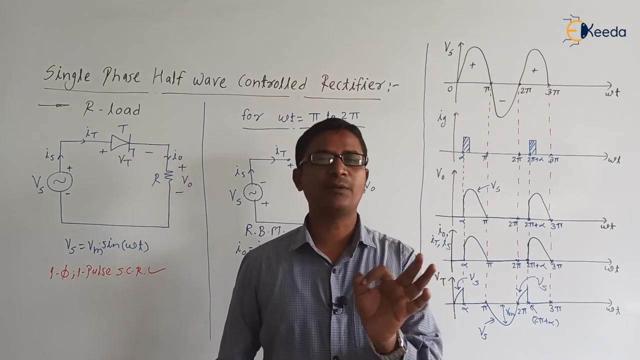 scr. okay. next, if the input supply frequency is 50 hertz. suppose if input supply frequency is 50 hertz, then what will be the output pulse frequency? right, input supply frequency is 50 hertz. the meaning is the input supply is completing 50 cycles in one second. okay, so in one second the 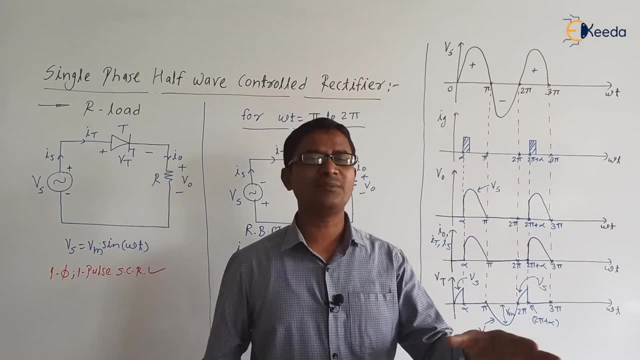 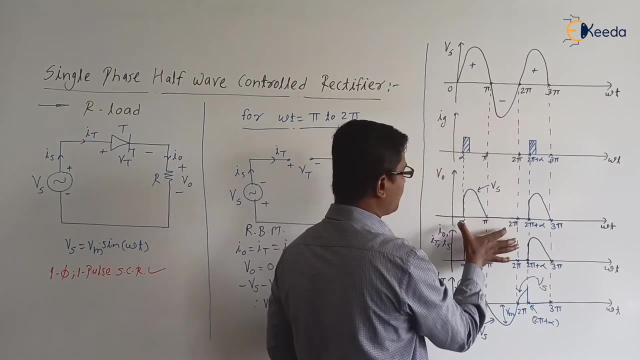 input supply is completing 50 cycles. okay, so that is the meaning of 50 hertz. okay, so what is the pulse frequency of the output voltage, as i said, corresponding to one input cycle? in the output we are getting only one pulse, so in one second, how many pulses we will be getting for? 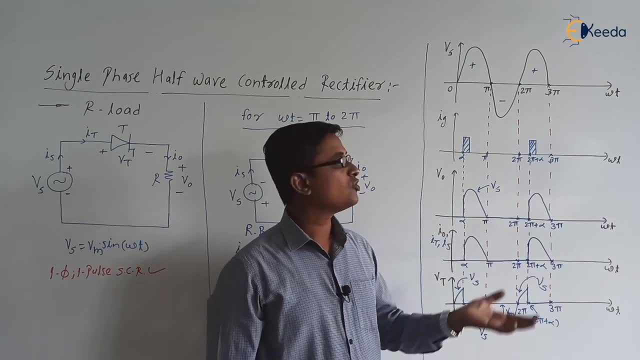 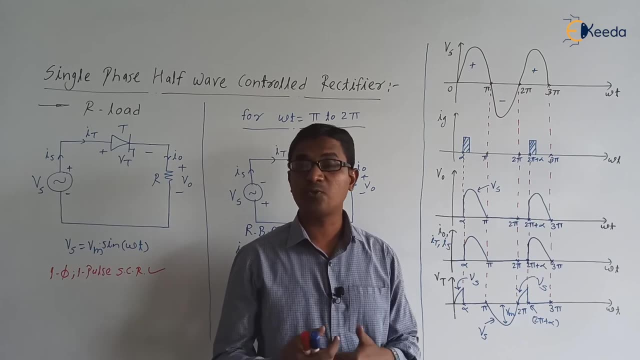 this v0 definitely will be getting the 50 pulses right. so for one cycle, whereas the one pulse, so for 50 cycles of the supply. we will be having 50 pulses in the output, okay, so what is the output pulse frequency? it is a 50 right. so please be careful, or please try to understand the output.